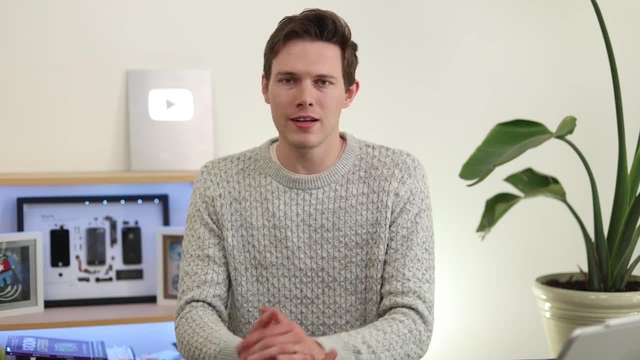 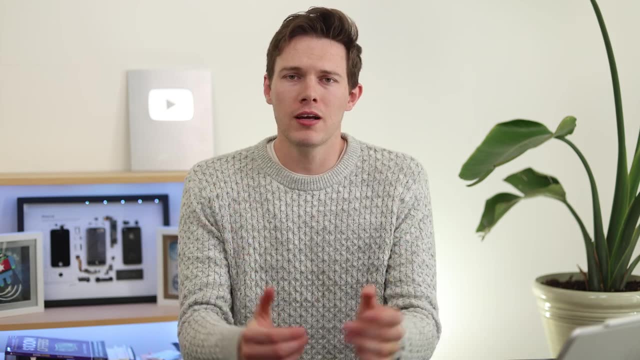 of a toss-up. WordPress has a lot going on, but there are ways to make it very easy. And then Webflow is slightly more advanced for some more in-depth customizations. So I want to start off on my laptop by showing you some of the different templates across these different platforms. 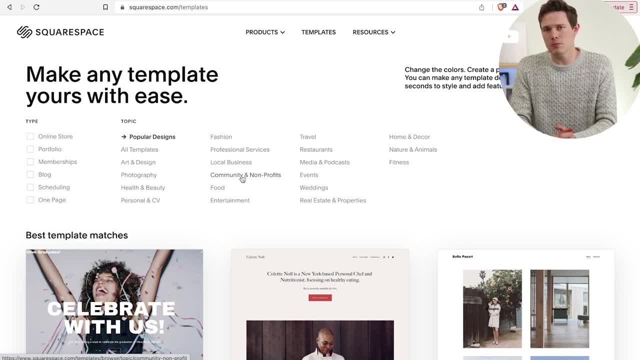 because ultimately, choosing the right template can have a massive impact on your website. It sort of acts as a launchpad and can save you a lot of work and make your website look really nice in the end. So I want to start off by showing you Squarespace, which has about a hundred different 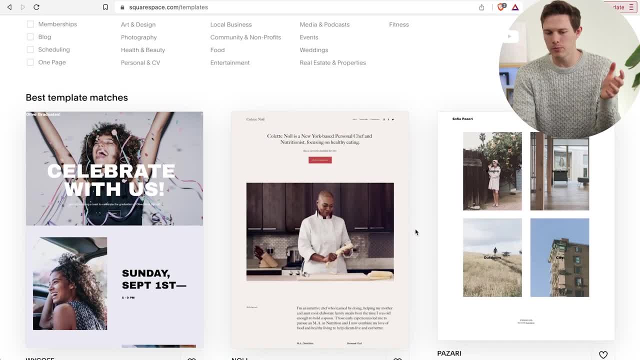 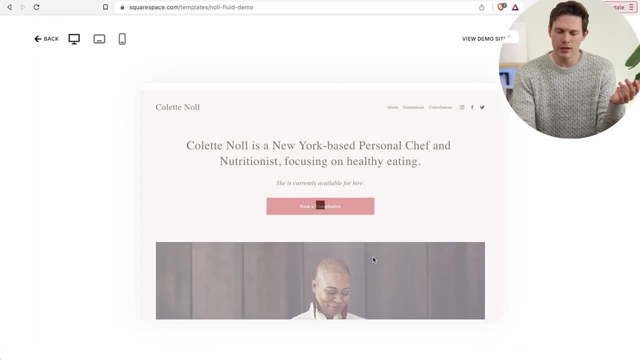 templates- slightly more than a hundred templates, And all of them are generally a little bit more minimal. They're all included with your plan, which is really nice, And you can look at any one of these, for example this one. if I say preview, it can show me that it's a robust website. 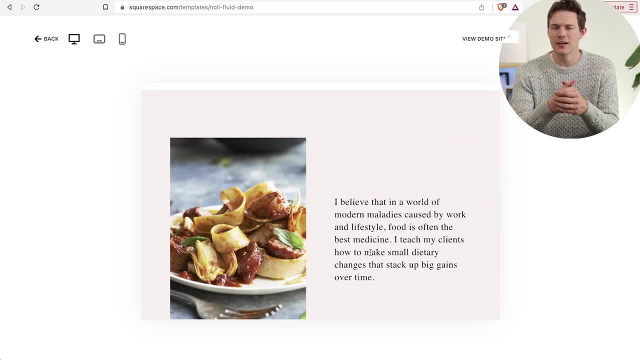 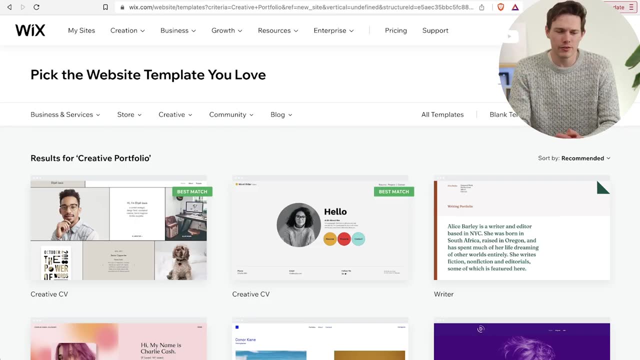 It looks really nice: minimal in design, but it's clean and elegant, And so you have a pretty good selection here. And that brings us into Wix, which has between 800 and, I believe, maybe even a thousand different templates. The number is always changing. 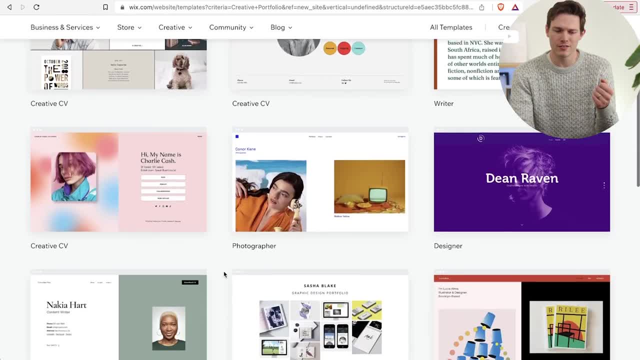 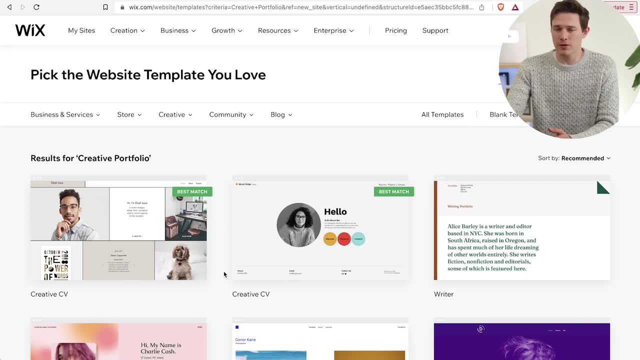 And these, once again, are all included, So you don't have to pay extra for these. but having that larger variety allows you to have more options within each category. So if you want to make a personal portfolio, or if you want to make an online store, each one of those you have. 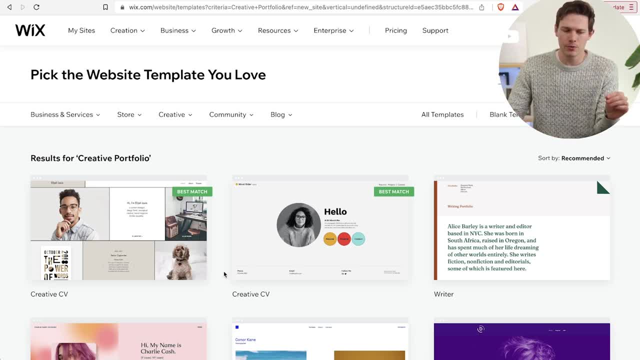 more options with that And in addition, when you're first setting up your Wix site, you do have two options. You can either create from a template or you can use Wix's AI to make the website for you. I generally like to go with the templates. I can kind of see the style ahead of time. 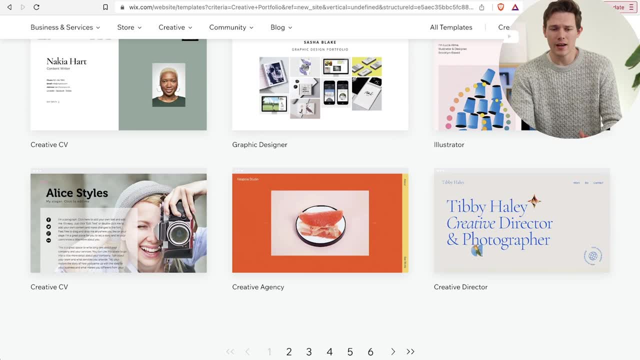 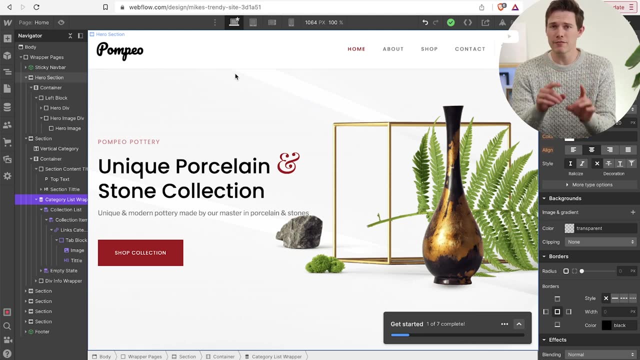 and it does a good job in my opinion. But moving along to the next one, being Webflow. Webflow has quite a few different templates. I believe they have on the order of 1500, but many of them you do have to pay for. Now, Webflow templates tend to have more animations in them, a lot more going on. 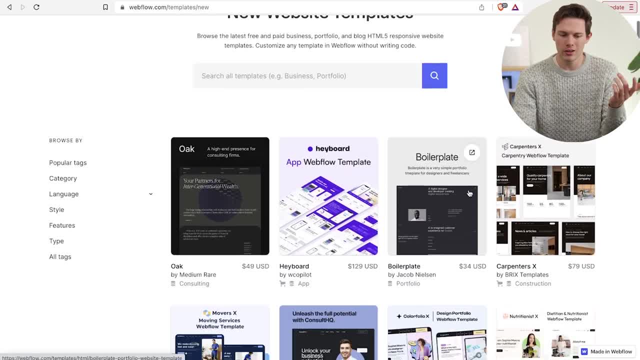 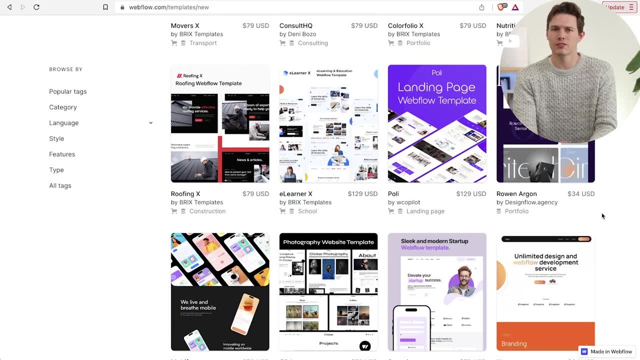 especially the ones that you do have to pay for. So you can see just the new ones right here. This one's like $130.. We've got $79.. A lot of them are $79 or $129. So it can be a little bit. 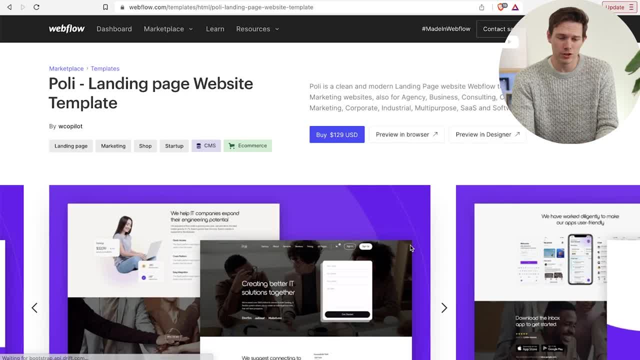 pricier, but we're going to have to pay for them. So we're going to have to pay for them, So we're. of course, you are getting a very robust web page just from the very beginning, not just one page. 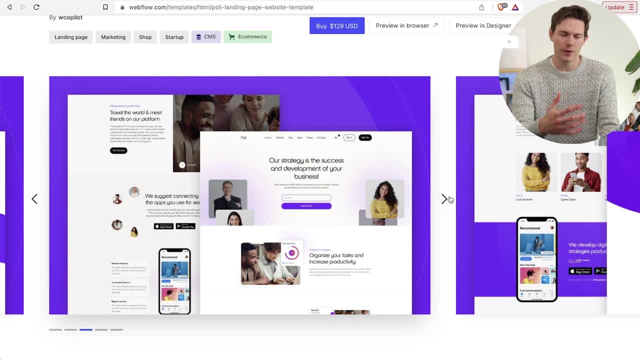 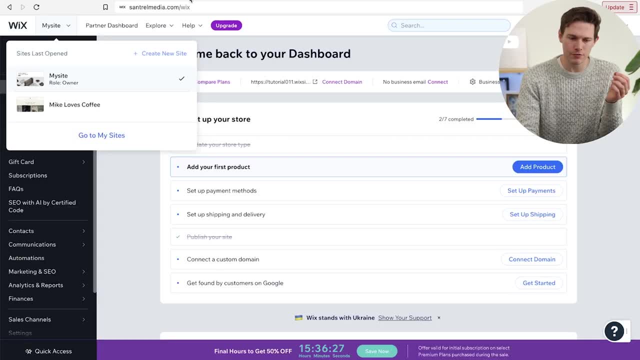 but your entire site And again it is kind of a trade-off. You will have to pay for this, but sometimes you can have some really cool animations on there. Moving on to the next category, This is going to be ease of use, So, as I close out of some of these different pages here, 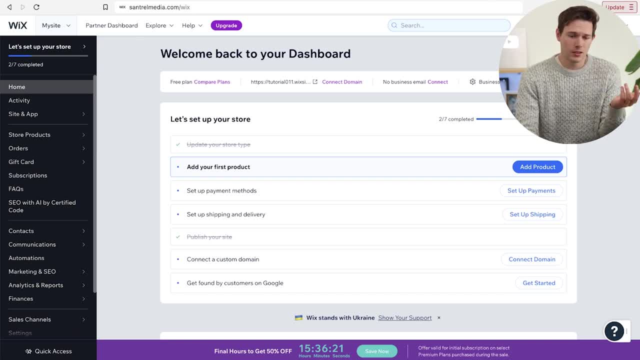 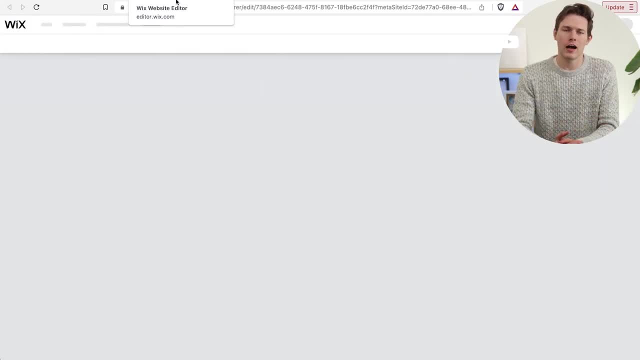 that we don't need anymore. you can see that Wix is really it's always been known as one of the easiest ones to use, but that doesn't mean it's like rudimentary, Like you do actually have a lot of flexibility here and you can customize your website in some pretty advanced ways, while 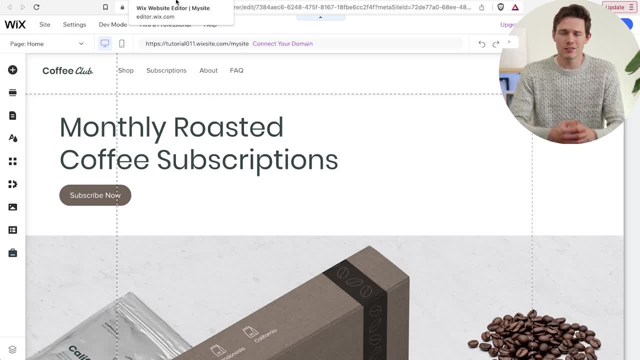 still having it nice and robust. a drag and drop editor that scales really well. I guess what I'm saying is: you can start off as an absolute beginner and make a nice looking website, or go on as an expert and make an incredible looking website using the same set of tools. So I've always really 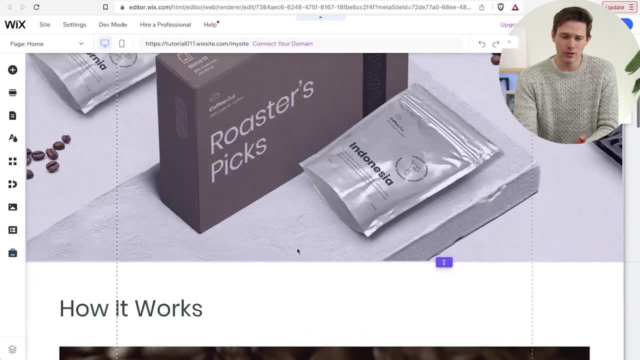 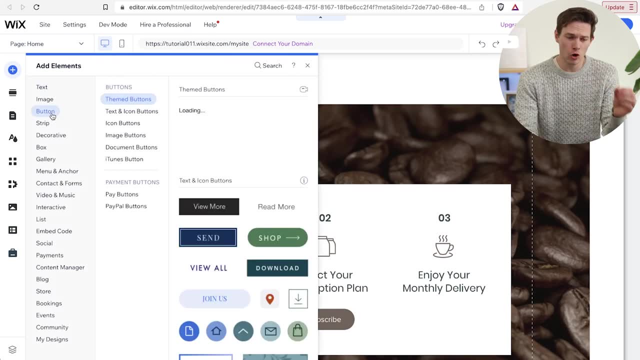 liked how they do that And within the editor it's really basic. As you go down, they highlight different sections just with your mouse and you can just click on the plus and add what they call elements. They have so many different elements on the left side that are pre-structured, So you don't have 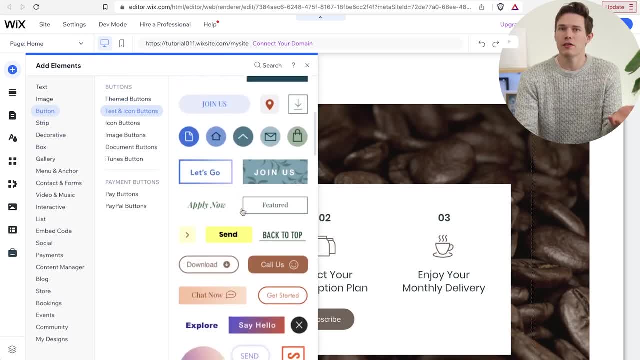 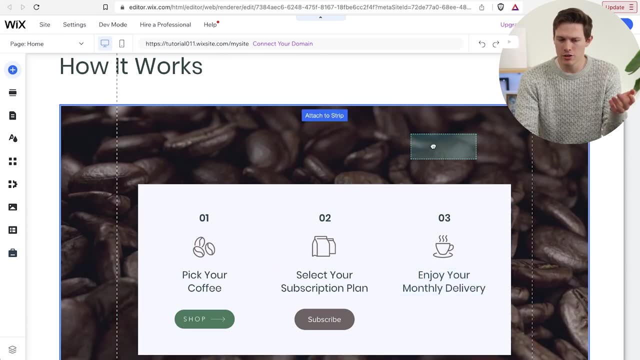 to format buttons nearly as much. For example, when you just go and see they have a lot of different ones like this. would take a little while to design that, but I can just click and drag that over and put it anywhere I want on my page. If I want a button right there I can put a button. 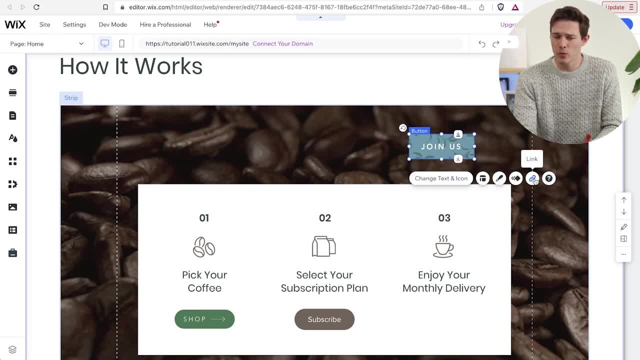 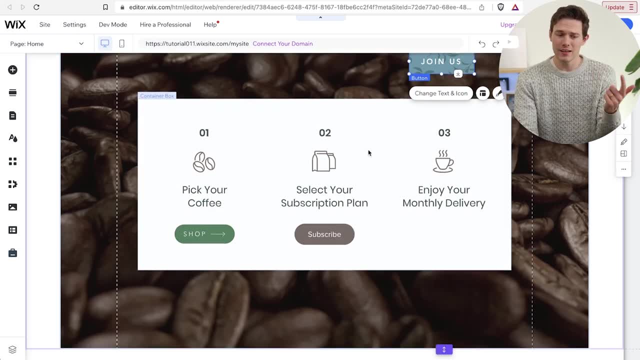 right there As far as editing goes. you can see everything right below there where it's going to link to what the icon is, what the text is. It's all super easy to edit And so very robust and very easy to edit. 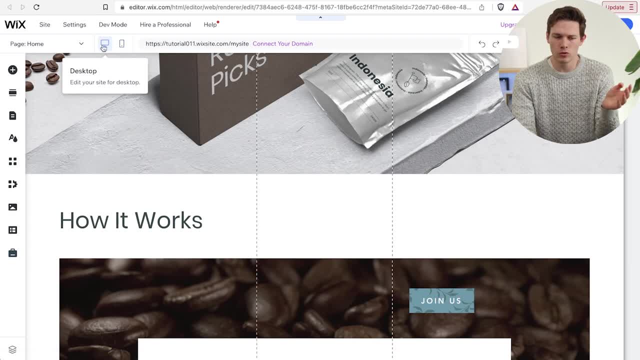 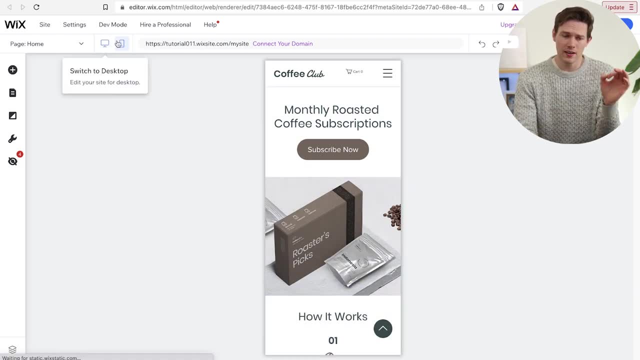 You might wonder what I mean by that. What I mean is, as you go over to like mobile, for example, your website doesn't break, It still looks pretty decent and everything is very responsive. So that's Wix. Now moving on to Squarespace, if we just click on edit for this website right here that I have, you can. 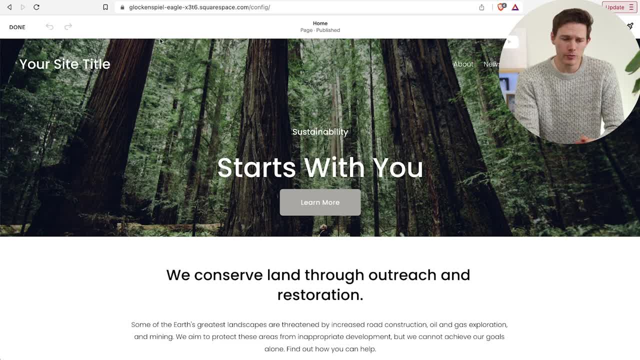 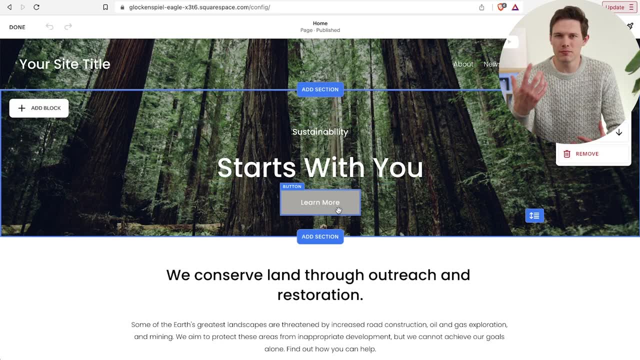 see that Squarespace actually changed quite a bit over the past couple of years. It used to be a lot more restrictive like. it used to be much harder to put things wherever you want, Whereas now it does kind of have a grid drag and drop style editor. So if I want this button to be over here, you can just. 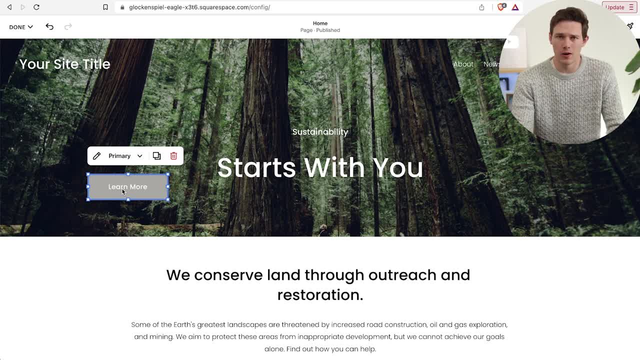 see, this grid kind of appears and I can put it over there and it works really well. Now, the reason they have that grid is to make it even more robust, so that you don't have to worry about a responsive design here, as things you know stretch and scale on different monitors: on TVs, on phones, tablets. 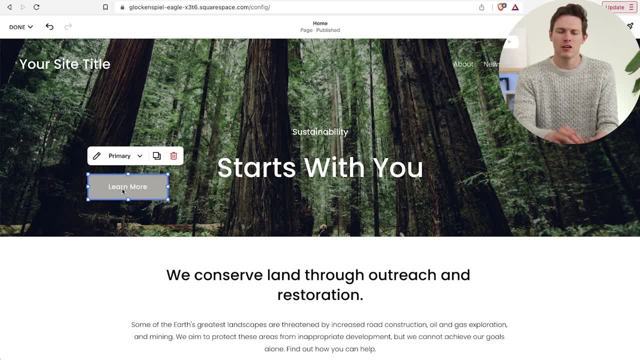 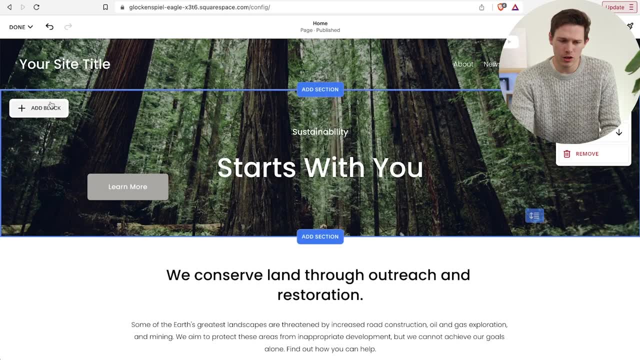 whatever, it should be able to handle that really well and keep things well arranged. So with that in mind, I really like how Squarespace has optimized their editor. When you want to add things, you can just go and click on add on, you know, on that specific block, And then you can go down and see that we 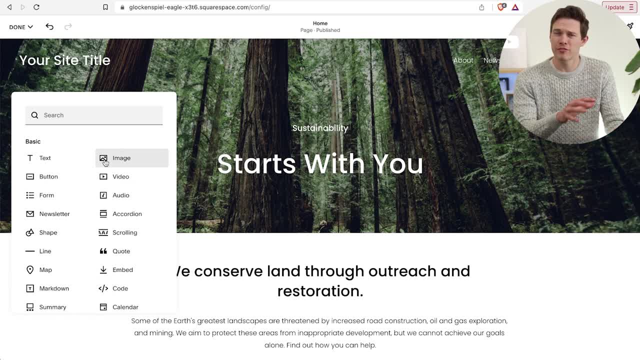 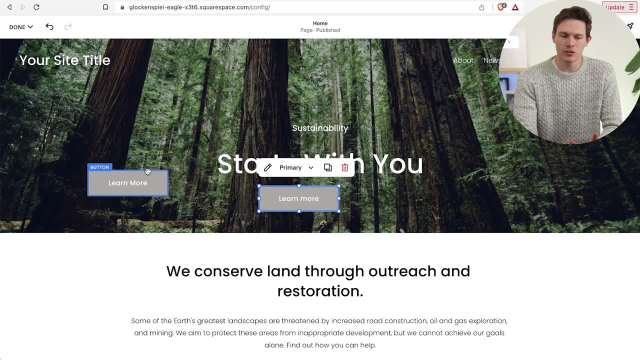 have again quite a few different things here, probably not quite as many pre-formatted elements as Wix has, But with that you do get really. you know simple, clean things: drag in a button and it's going to match the previous button, Like there is this style that you're going to have. 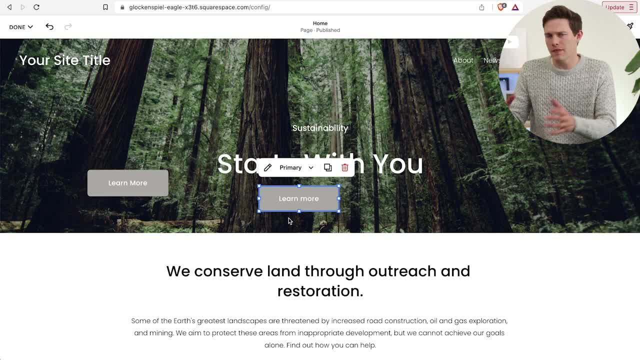 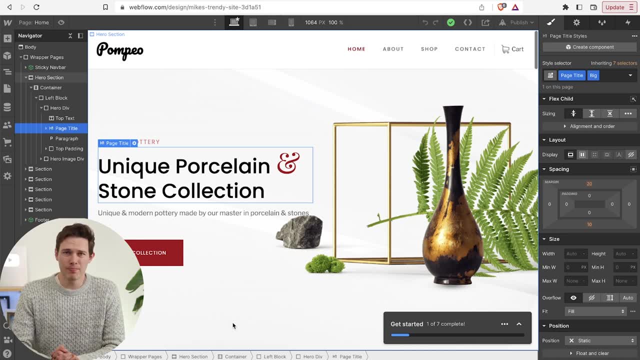 uniformly across your website. So less customization and a lot more uniformity and also ease of use when you're doing that. So then going over to Webflow, this one is definitely the most difficult to learn for beginners, But, like I said, I have a tutorial to show you how to do that. 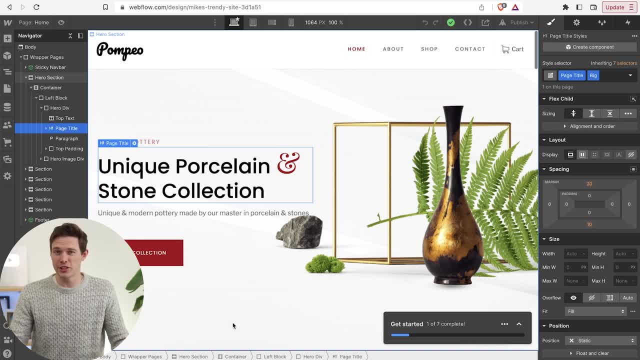 And with this you're getting an incredible amount of freedom. You can change a lot about all these different elements on here, And so with that you can have great animations on your website. You can have exactly like, perfectly located graphics, and you can still make it very responsive. 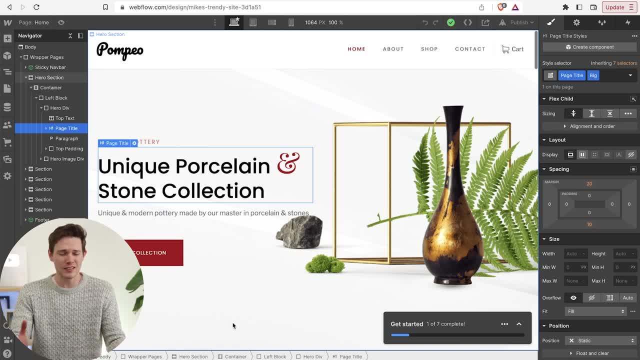 with different breakpoints set up as you make the website. But, as you can see on the dashboard right here, if it seems intimidating, that makes perfect sense, because this is definitely meant for somebody who is looking to do a lot more with their website, a lot more customization On the right side we can. 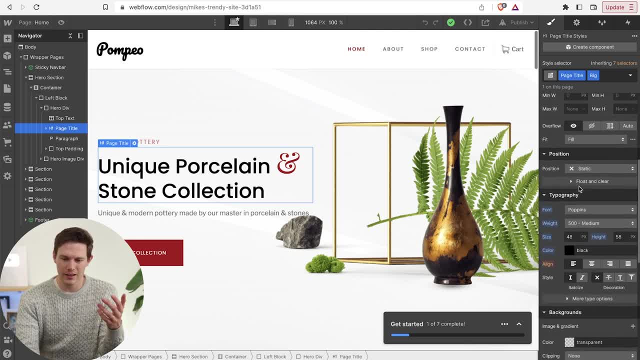 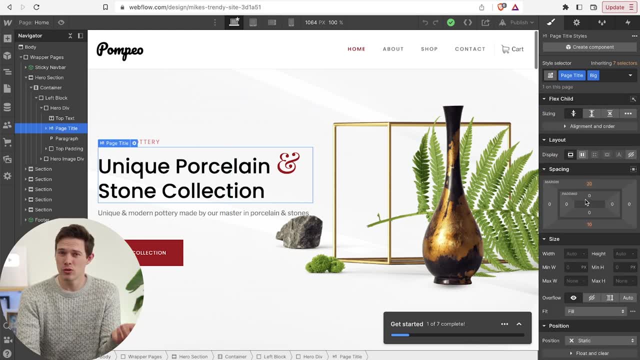 customize everything on here from like location and color and like it looks a lot more like an Adobe Photoshop style layout here. And personally, like once you get used to it, I really do like this. But for beginners like I do, caution, you trust me, this is, it's a little bit tricky. Now Webflow at. 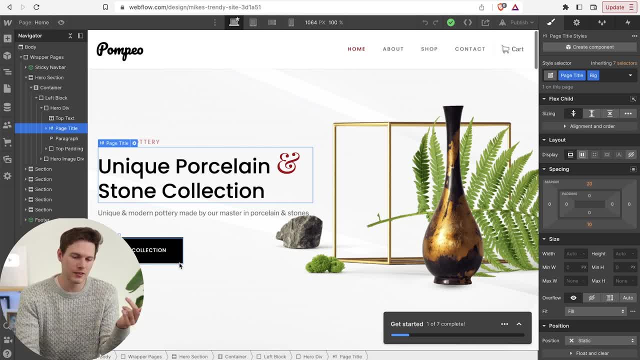 the same time, does you know, give you tutorials when you start. they show you how to make different buttons and add things to different collections and make a new button that matches the old button, So editing your entire website. you do have some really powerful tools there, Like, for example, 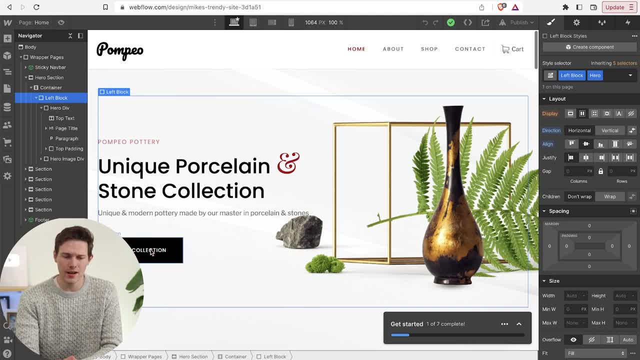 I have all of my buttons on this website set up with the same style class as, like this one right here. I could just change the color of that and every button on my website will change. Great way to edit websites. makes it really easy when you have larger websites. Going on to the fourth one, 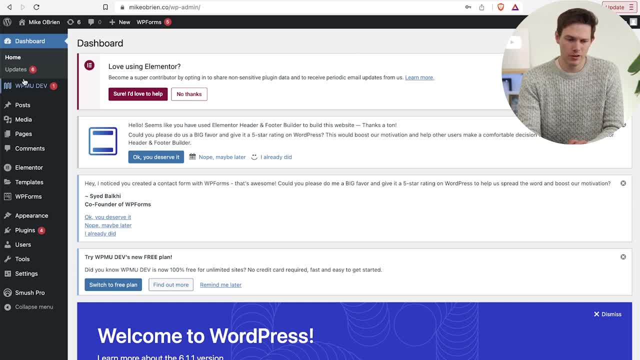 this is actually WordPress, As you can see. I have an example site right here that has a lot of updates. I didn't do yet, But if we go to pages, I'll just show you the quick editor. What we like to use is called Elementor. It's one of the easiest ways to make a WordPress website where you have 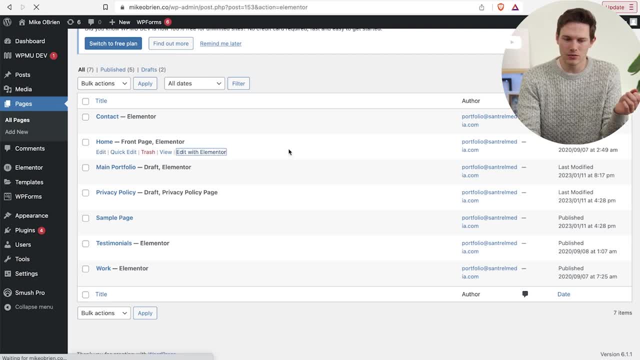 so if I go to, for example, the homepage, I can edit this with Elementor. So here we are on the Elementor interface And, as you can see, it's kind of like a combination of Wix and Squarespace. 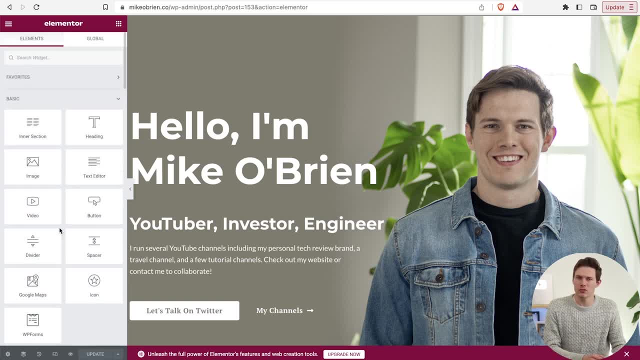 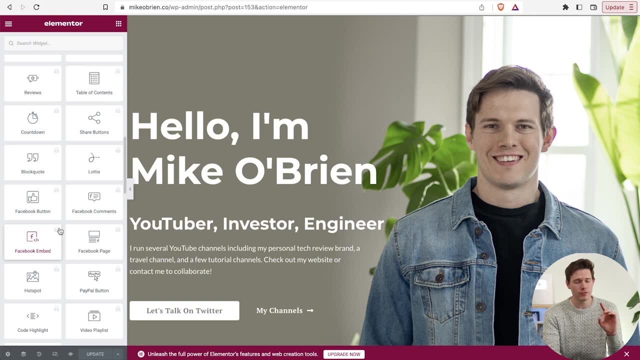 we have a lot going on in the left side. They're not pre formatted like we saw on Wix, But we do have an incredible amount of elements we can add. Some of them are very advanced as well. Some of them are also limited to Elementor Pro, Because so far, setting up this right here is pretty much 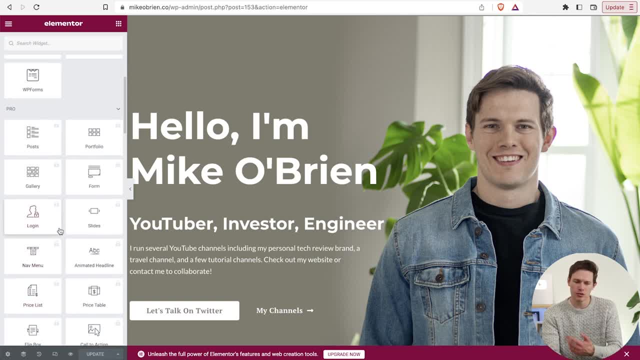 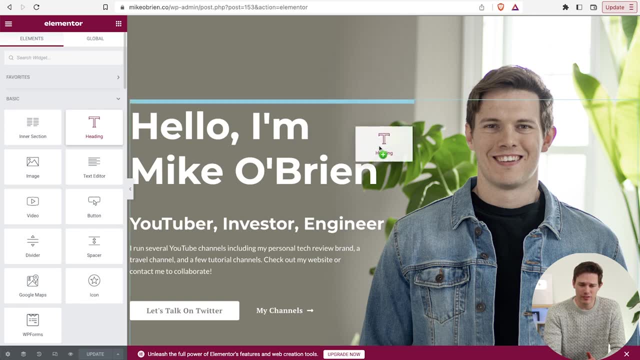 free right, Like we haven't. I'll talk about prices later on, But Elementor Pro is an option you could upgrade, but still a very affordable option, And otherwise if you want to add, for example, like a heading, you just click and drag that. this one is not necessarily a free form. 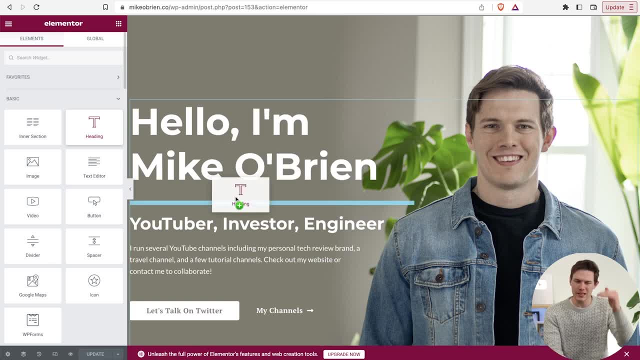 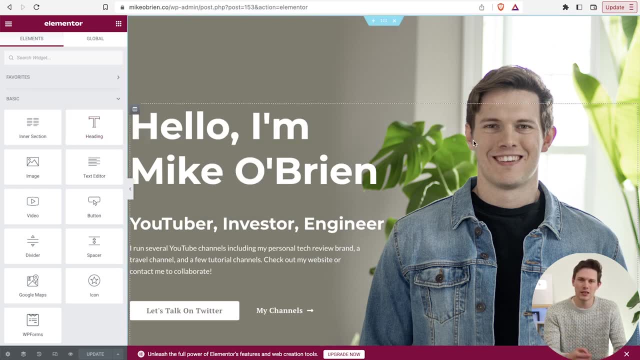 editor. like we saw in Wix and Squarespace, this one is kind of based on like reference to other elements, So you can put it below that one. you can't just like plop it over here that it doesn't really allow that. Now, the benefit with WordPress here is that you're not confined to using this. 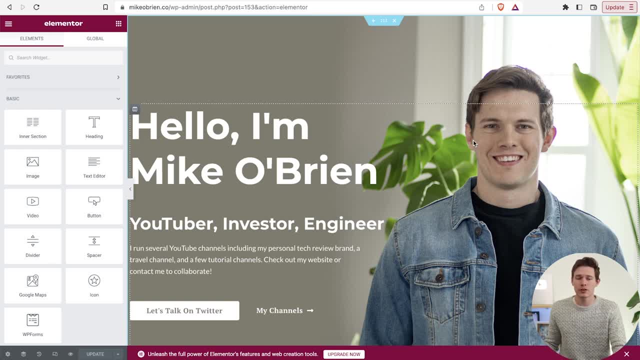 theme, which has a set amount of templates, or this website builder, which has a set, you know, constraints. here you can choose different ones, like Divi, for example, or there's a lot of other ones out there. We also have a tutorial if you want to use Divi instead, as really I really do. 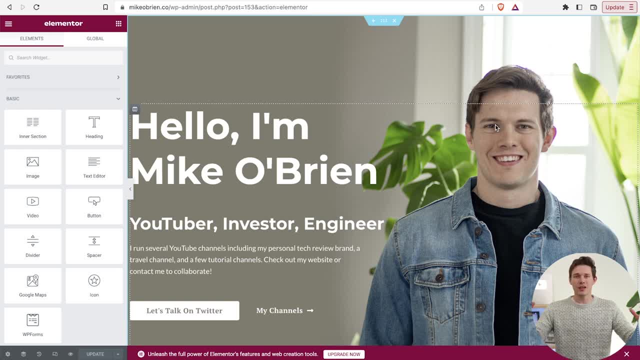 like Divi. it's kind of a toss up between Elementor and Divi for me. But, moving on to the next category, if you want to actually start making money with your website, of course lead generation and affiliate marketing is great. But if you want to sell physical or digital products, which one of 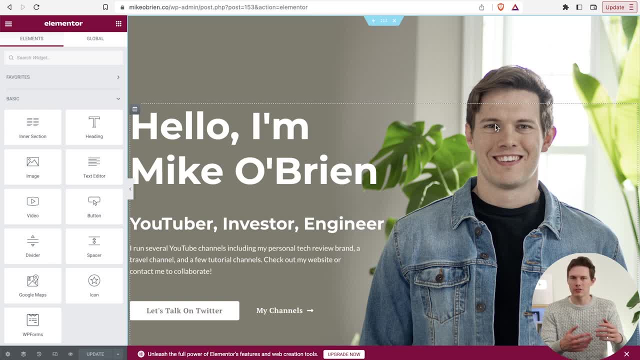 these is actually the best. Well, since we're on WordPress right now, I'll explain how this works. So what WordPress kind of operates is. you have a basic infrastructure and you add plugins on top. So you can add a plugin like Elementor to make it easy to edit. you can add a plugin to make SEO. 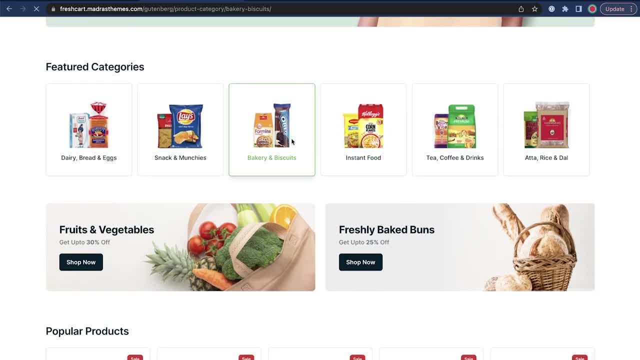 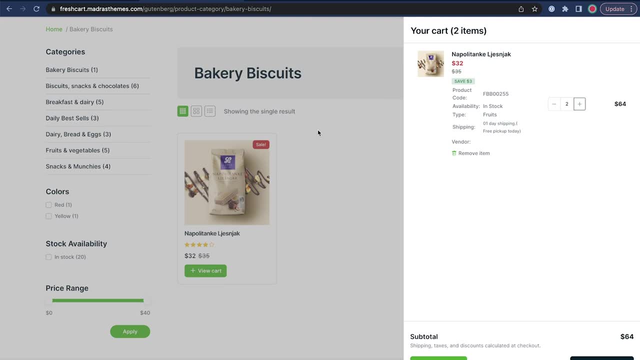 easy. you can add another plugin called WooCommerce to make online sales very, very easy. This is great for managing inventory. it has a lot of different options for types of products. you can sell not just digital products and physical products, but drop shipped products or gift cards. 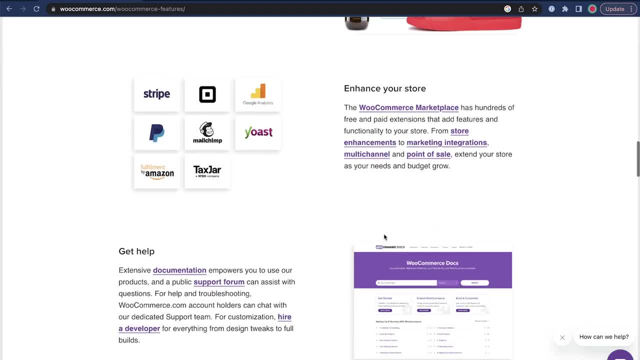 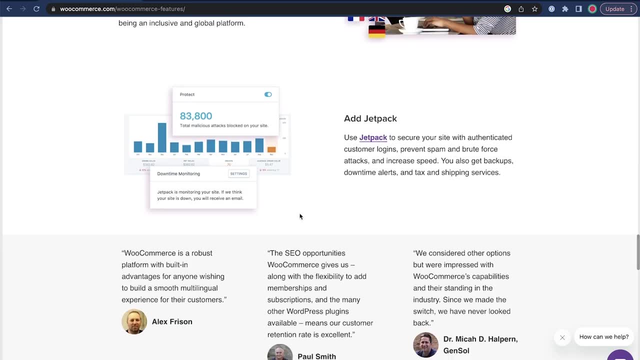 with different styles, where you can say you get discounts on certain items if you buy only like two of them. Like, it's very, very flexible And you can really do a lot with that. So WooCommerce, I mean it's hard to argue against it, it's really easy to use And it's very, very robust. 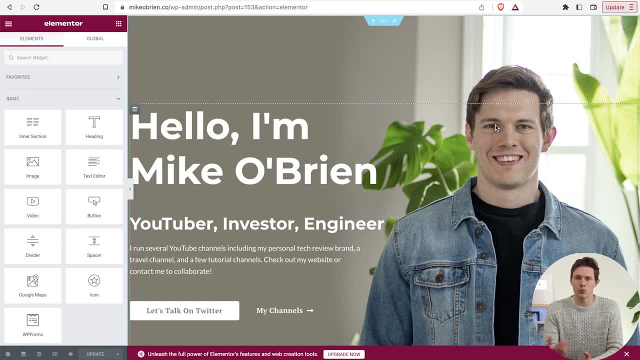 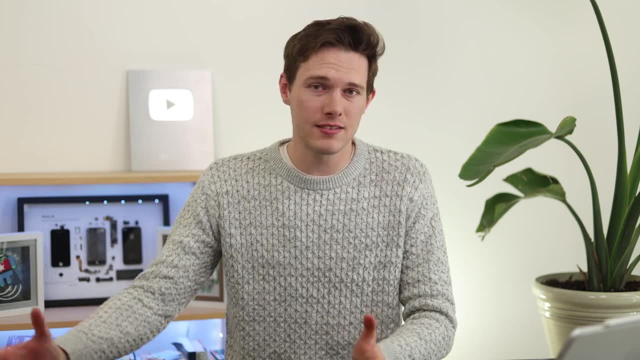 you just have to get through making the rest of your WordPress website And, once you have it set up, like tons and tons of functionality there, And really the big benefit here is that it is highly scalable. So you can start off with a really tiny website: one page, one product and 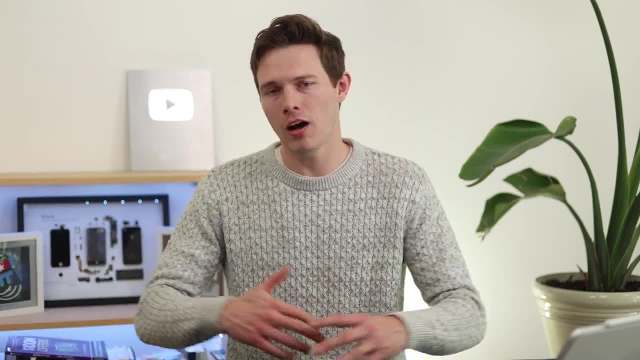 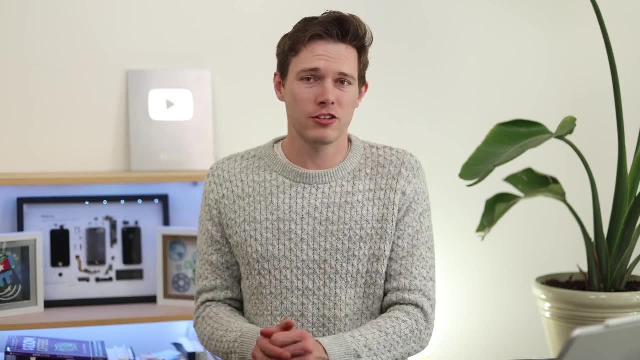 up to many, many different pages, tons of blog articles, tons of products, a massive inventory and a big library of products, And it scales perfectly, which is why WordPress powers such a huge portion of the internet. Moving on to Webflow: In the past, to be honest, I haven't 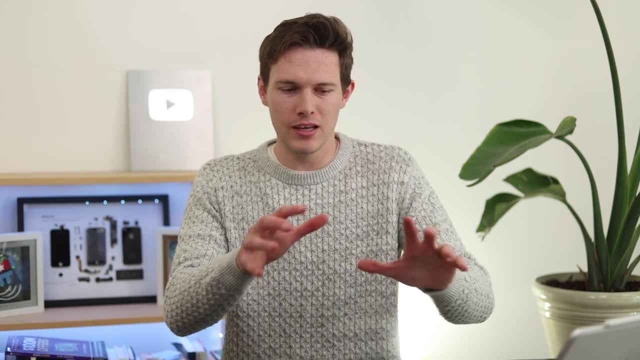 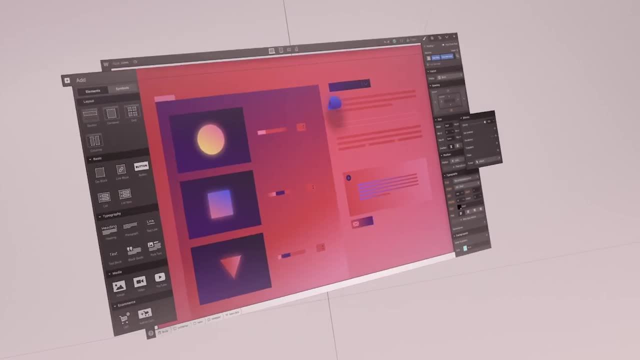 actually sold things on Webflow. I just always used it to make like more advanced websites like this, But for whatever reason, I never ended up selling things on them. But regardless, you can do it. you can integrate with like Shopify, for example, and sell things on here. It's probably. 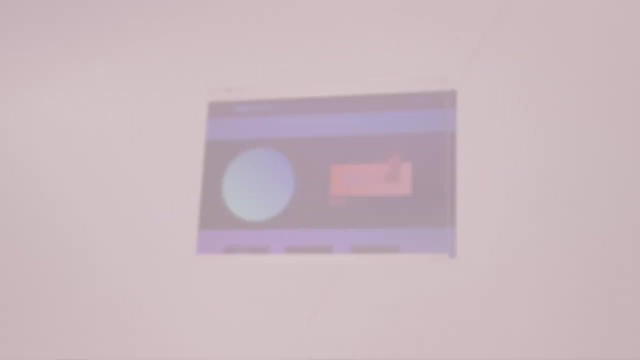 not my favorite website, but it's probably one of the best websites I've ever used And I think it's my first choice for an e commerce website, especially a beginner. But moving on to the next two being Squarespace and Wix. Now Squarespace has e commerce plans available and built in store. 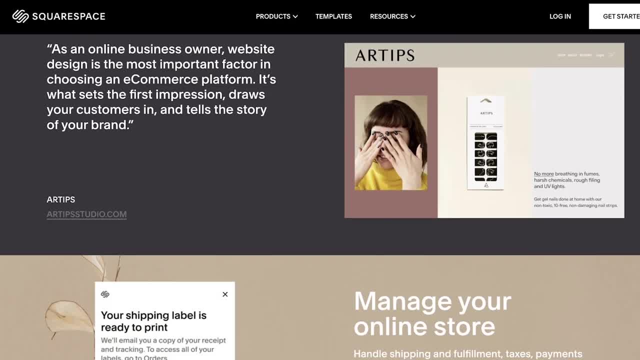 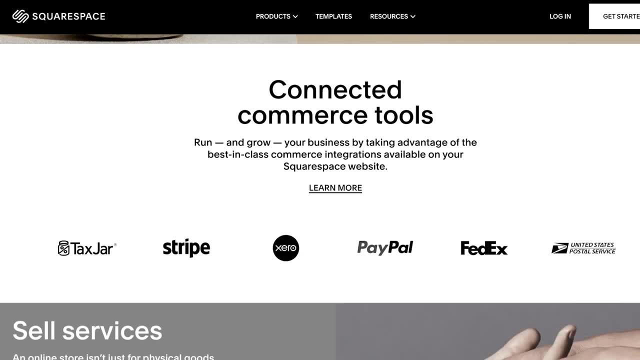 functionality, So you don't have to get extra plugins. you don't have to look for different things, It's automatically baked in here. they have basic inventory management. they have shipping settings. you can choose different product options, like physical products or you. 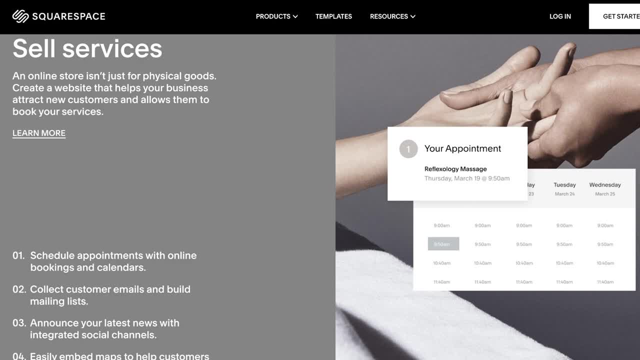 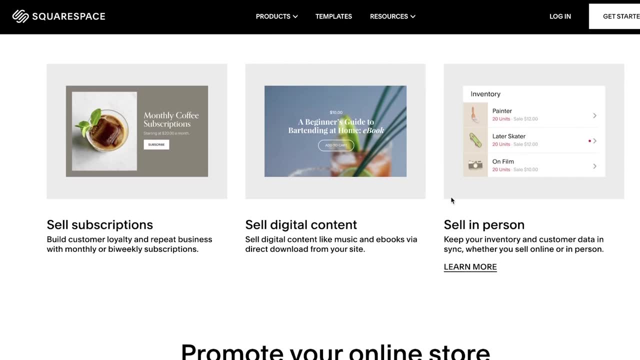 know different types of digital products. As far as fees go, there are transaction fees for the lowest e commerce plan But depending on how much you're selling, you can upgrade to a higher e commerce plan and you would get rid of those fees. And as far as payment gateways go, 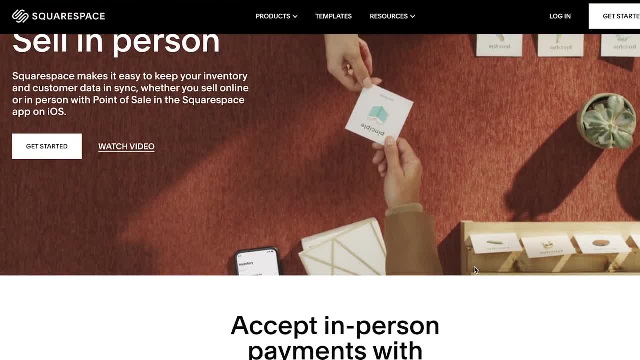 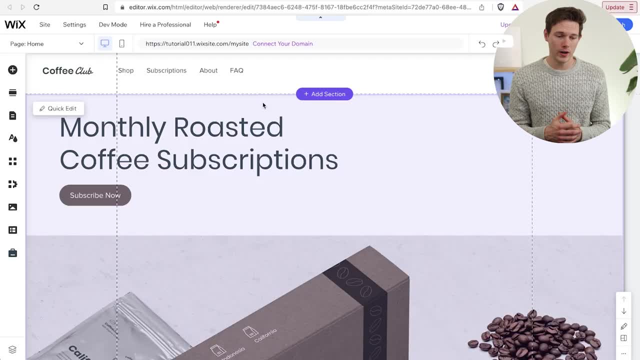 there are Stripe, PayPal and Apple Pay. Those are the main ones that are supported here, which is why I think this is great for like influencers trying to sell some merch or something like that, And then, of course, we have Wix. Setting this up is super. 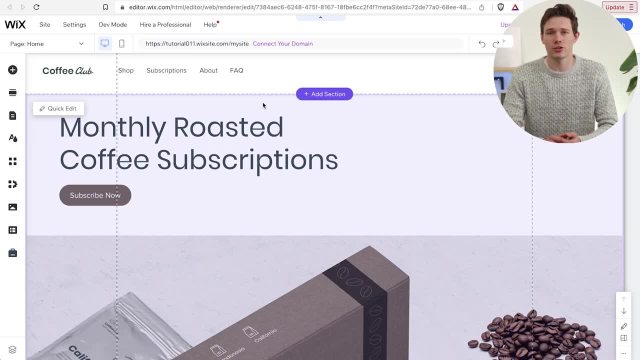 straightforward. There are e commerce plans available with built in store functionality And you can have a lot of apps on here. One of the big benefits of using Wix is they have their entire app market. So if you just go to add apps, there are a lot of. 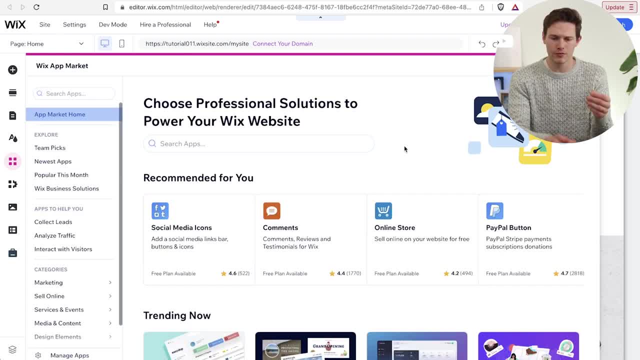 different integrations here, which can make this a very viable option for drop shipping or adding different shipping functionalities to. you know, send SMS notifications, for example, to whoever buys things on your store. And as far as payment gateways, it supports a ton of them, like PayPal. 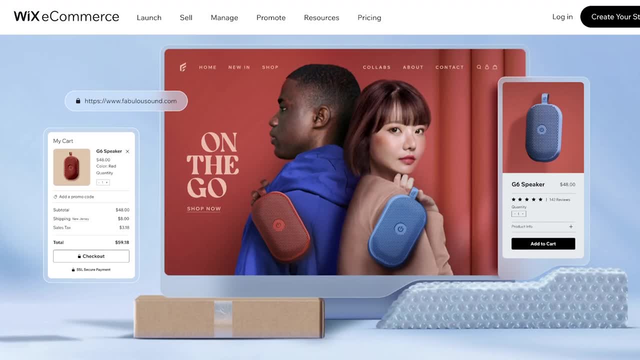 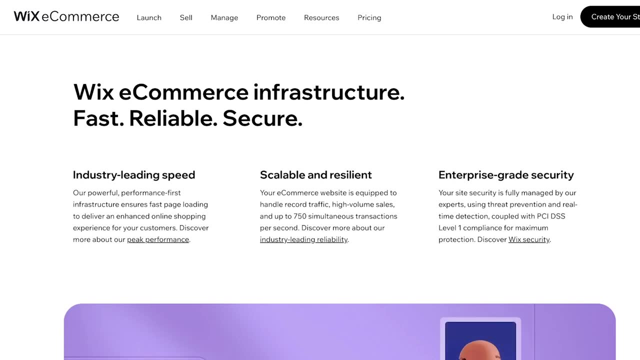 and Stripe and several others as well. But as far as fees go, the benefit here is: Wix doesn't actually charge transaction fees, But the payment gateways actually might, of course, if you're using Stripe, for example, I think the credit card fee on there is a couple percent, Of course. 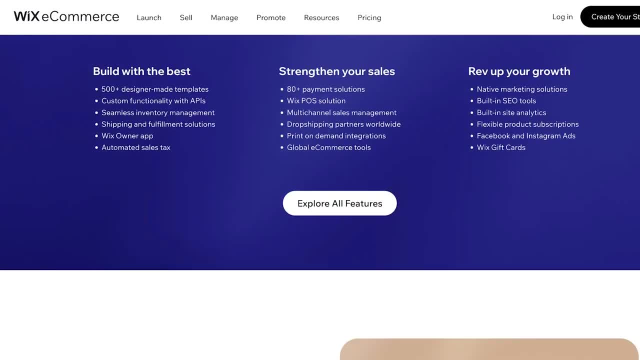 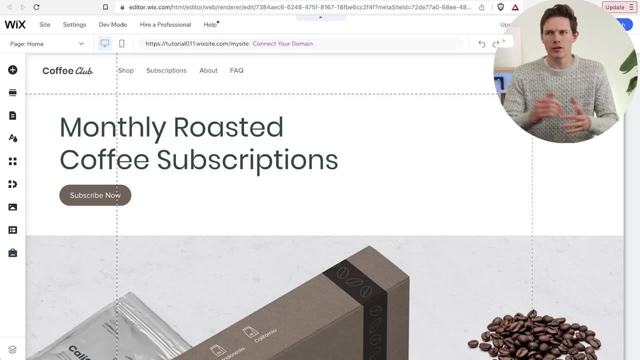 I said, Wix has inventory management, shipping and tax settings. they've got different products options And they have some abandoned cart recovery features as well to kind of improve your conversions. So generally like to review the scalability of Wix. it's great for obviously. 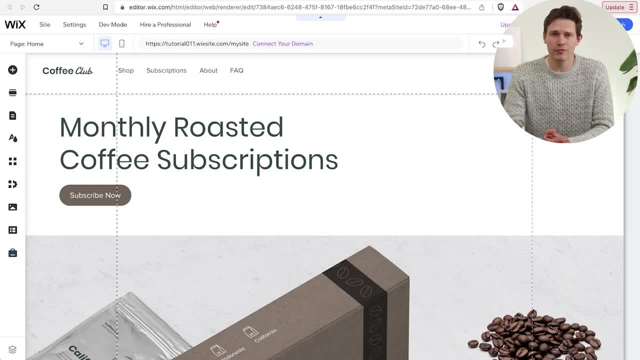 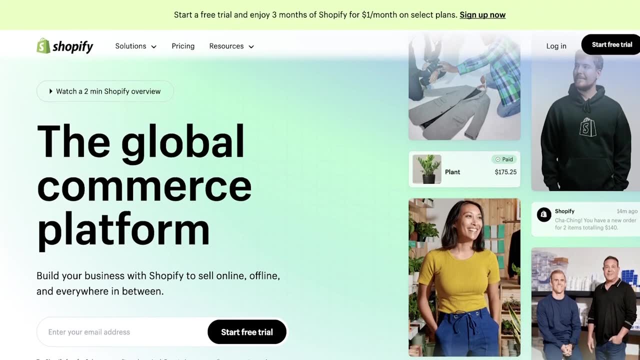 single product websites, But it can also scale up pretty far to have quite a large library, And Wix can really be used by the pros as well as the beginners. Now- although I didn't compare it in the rest of this video- when we're talking about e commerce, obviously Shopify is an absolute. 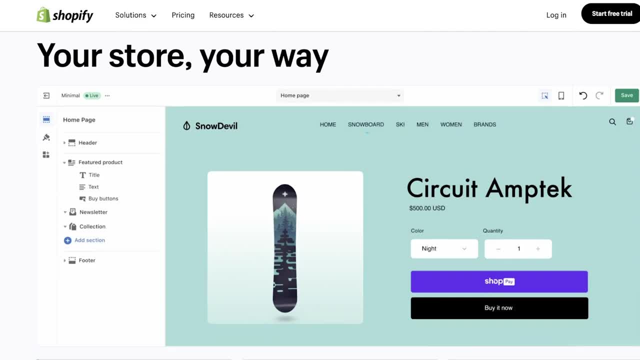 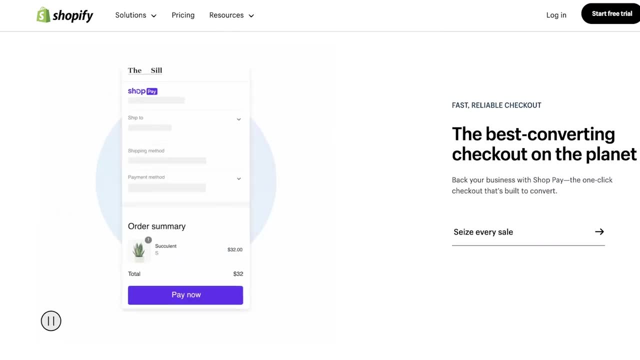 giant in this space and has a ton of functionality. So if you only care about e commerce, I recommend checking that one out. I didn't include them in this video because these are. these are website builders that you can use to build any website but also sell things on where Shopify if you're. 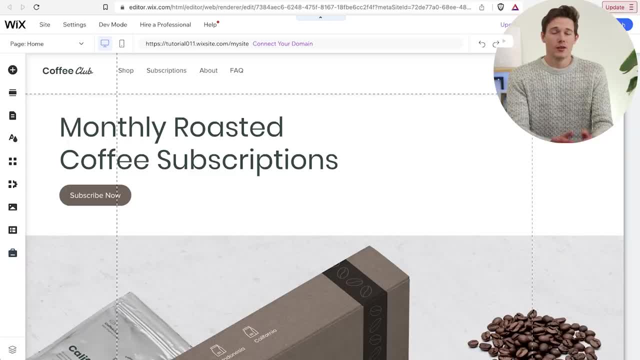 not selling things on there. I don't really know why you'd want to even use that. Next up, we have SEO, which stands for search engine optimization. Essentially, how easy is it for you to start ranking on Google with any of these? Since we are on Wix right now, I want to start off by talking. 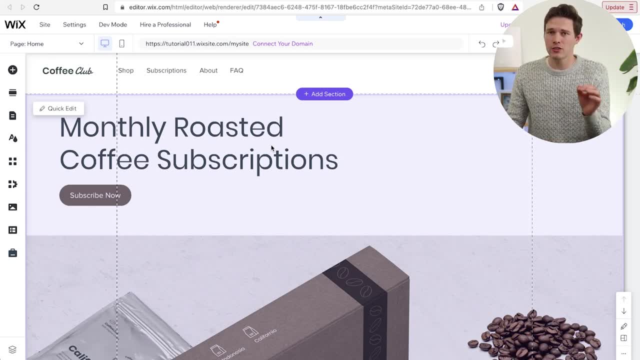 about. one of my favorite features out of all four of these is actually with Wix. they have something called SEO wizard which walks you through, step by step, different optimizations that it finds that you can do across your entire website to make sure that you are optimized to rank on Google And 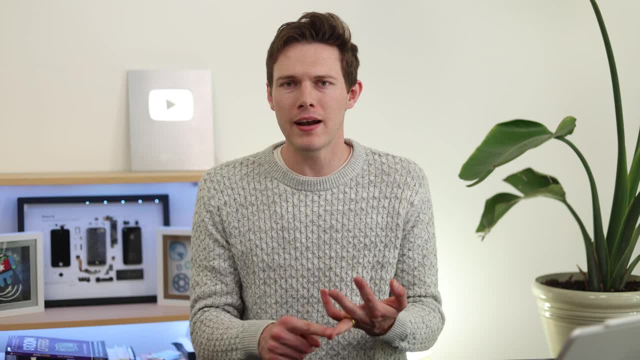 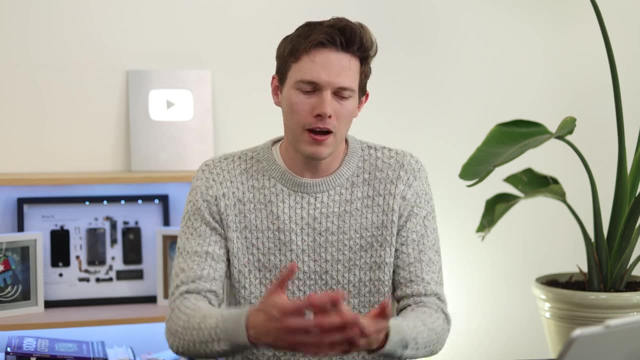 these are things like different alt text or choosing the right titles and and meta descriptions on different pages And, of course, just general website of health and hygiene in general. that I find works really well. So Wix gives you a lot of flexibility in how you design your site. 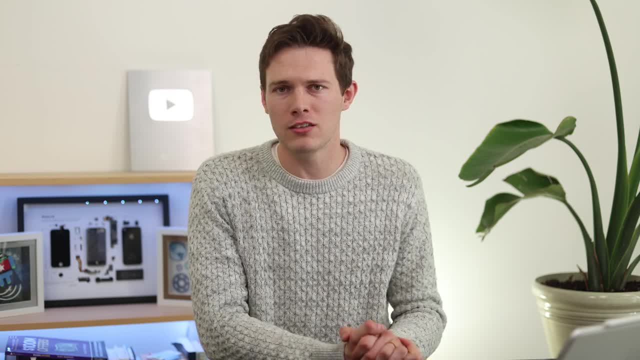 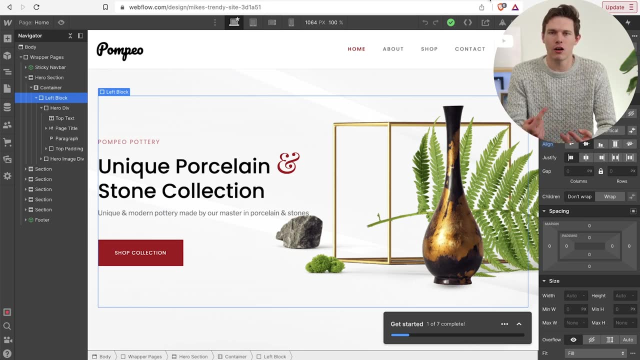 but then makes it super easy to go to one spot, use the SEO wizard and optimize your website. Then, of course, going to Webflow. SEO is pretty reasonable here. you're able to add meta descriptions and customize URLs and basic things like that alt text as well, So it works pretty. 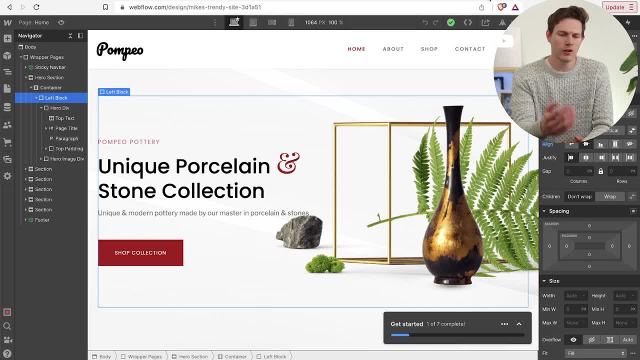 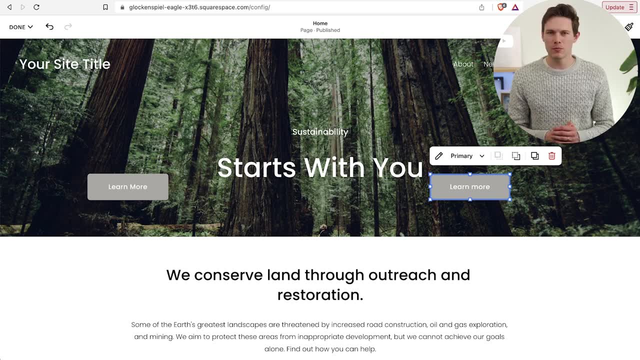 well, Not my first choice for making it easy to do SEO, but certainly possible to do on here. Then, as far as Squarespace goes, there's some pretty basic SEO tools. it's a little bit more limited compared to the competitors on here, But if you look at any of 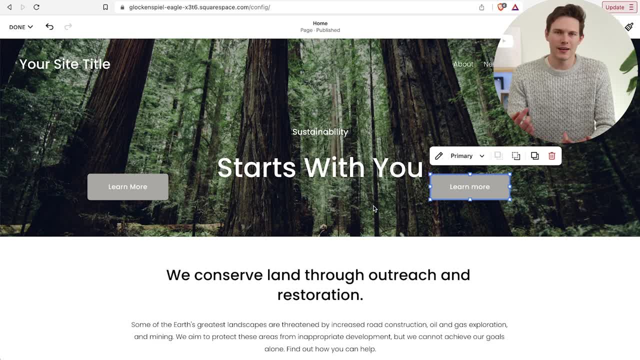 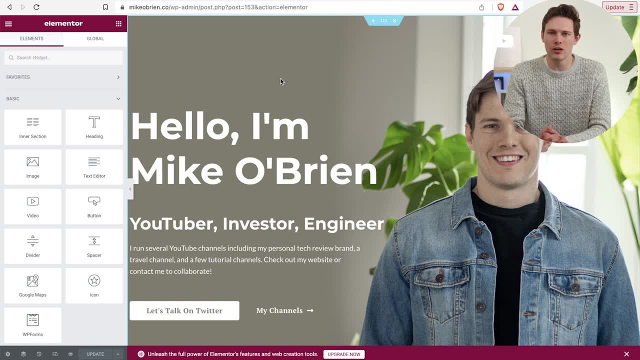 any individual page or element. you can optimize it, you can add, you know, meta descriptions and things like that for different pages. But really the king here has to be WordPress, where WordPress is giving you. like I said, if you use another plugin, this one's called Yoast SEO- it can do a. 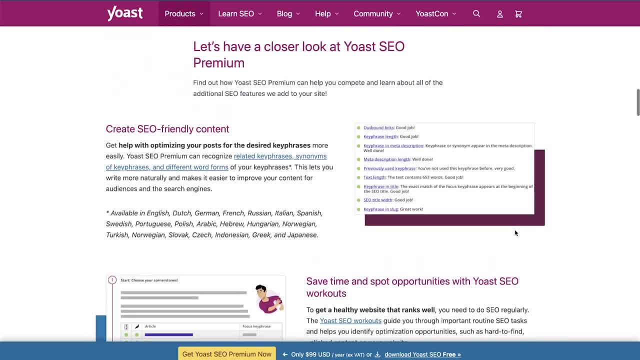 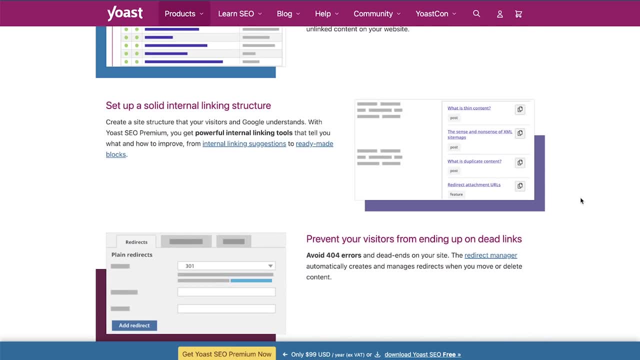 lot of what we saw, kind of similar to Wix, where it gives you like a checklist and walks you through And this can help you really optimize each of your blog posts. That's really where I've used Yoast SEO the most to make sure that, of course, the meta stuff like description and tags and title. 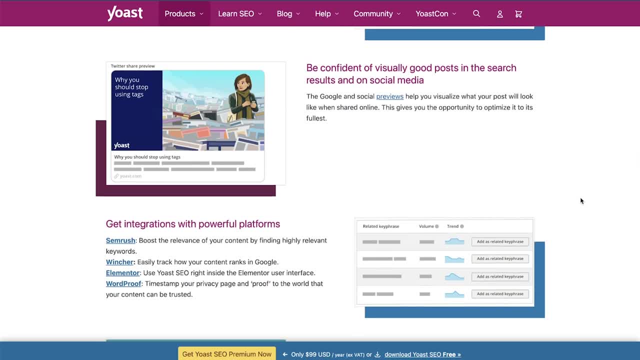 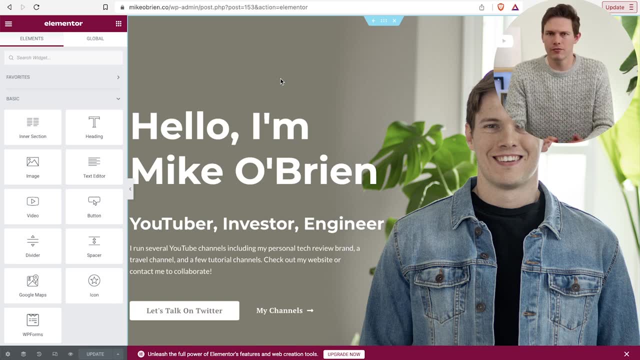 but also it'll kind of read through your blog and let you know if you use the keyword enough, not enough, too much and basic things like that, Actually not basic, pretty advanced things like that, Very cool. There's also like a free version as well as a paid version of that. 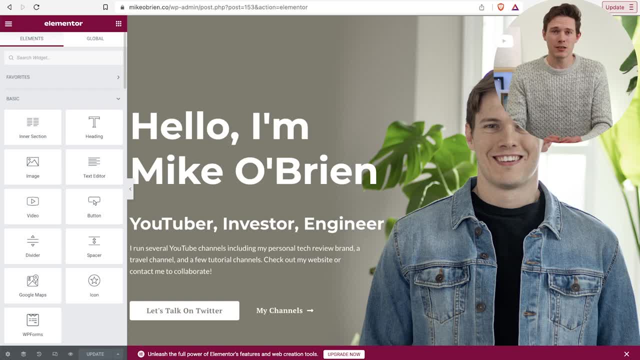 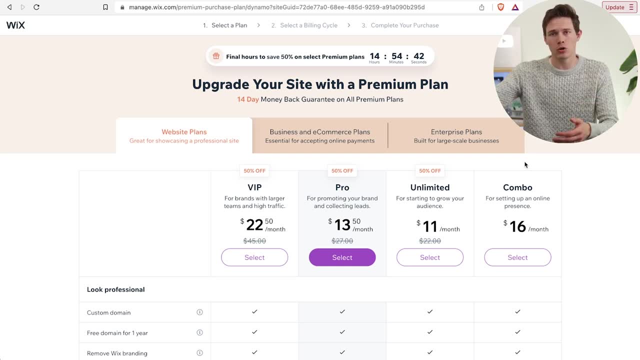 which kind of leads me into the next topic, which is pricing and plans. Now, looking at the pricing, starting off with Wix, Wix is by far the cheapest option, but could be a more expensive one as well, So it scales up really well. like I said, with the same websites you can actually start off for. 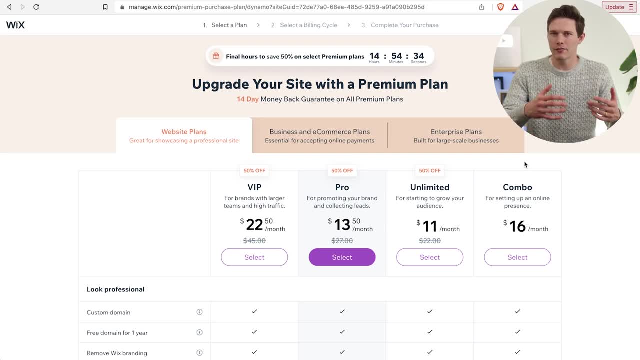 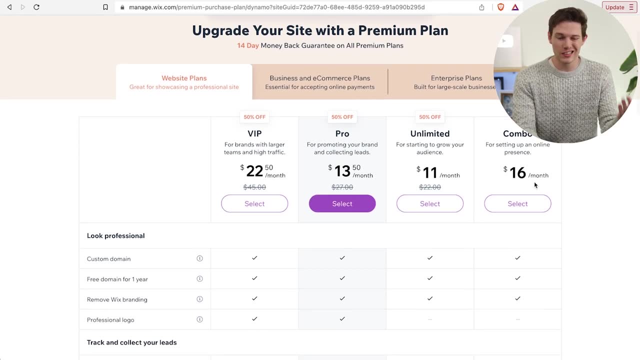 free. There are, of course, different branded, like there's limitations, You can't have your own domain and stuff like that, but for free that's really really impressive. And then from there you can upgrade to $16 a month or even $11 a month, as you can see right here, and really get. 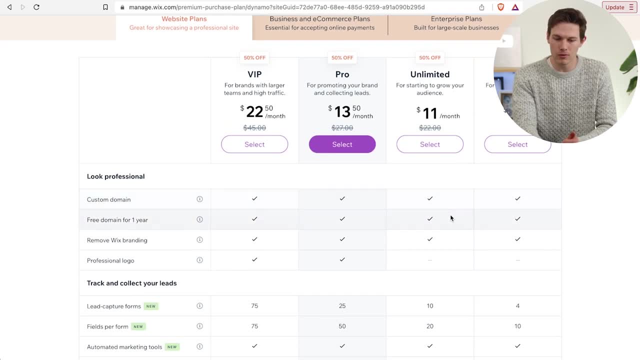 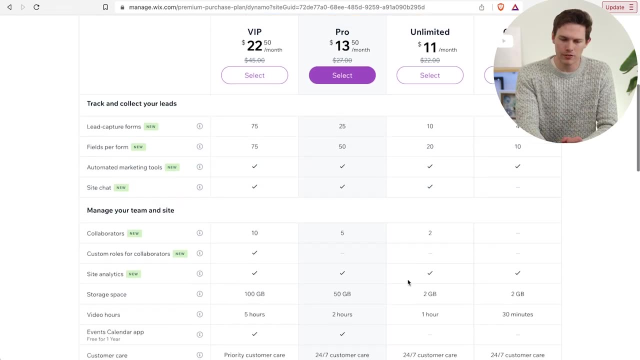 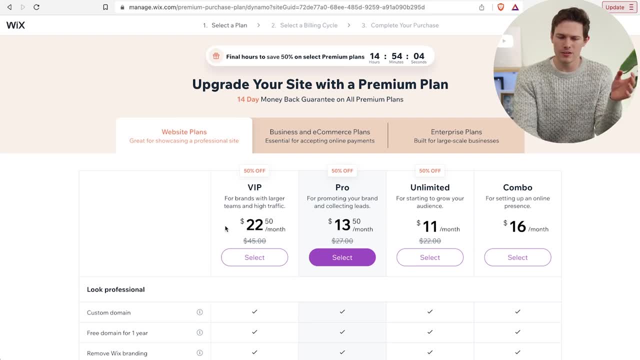 which is really impressive. And then you can upgrade to $16 a month, which is really impressive- Very impressive that you have that. Now this scales up, as you can see, to $22.50 a month. It looks like there's actually a pretty substantial sale right now. Usually it's $45 a month And there 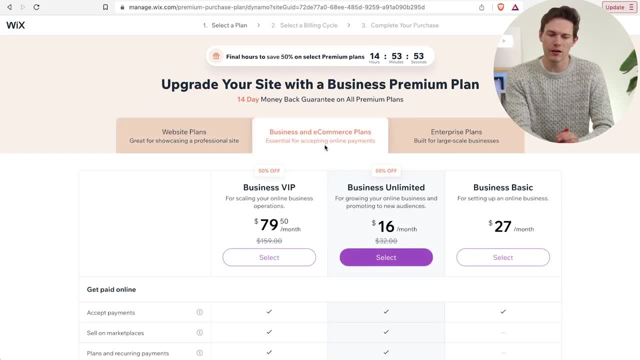 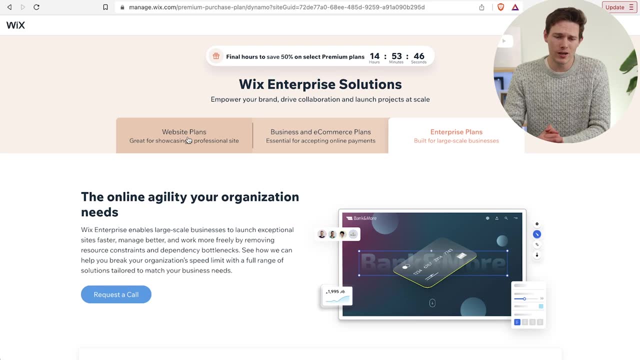 are also business and e-commerce plans. So if you want to sell things on there, quite a few different options here, And there are enterprise plans as well because, like I said, you can scale this up and pros can really use Wix as well. So then, of course, going over to Squarespace, the pricing- 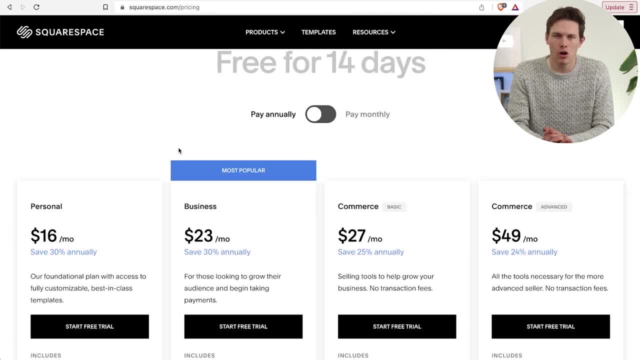 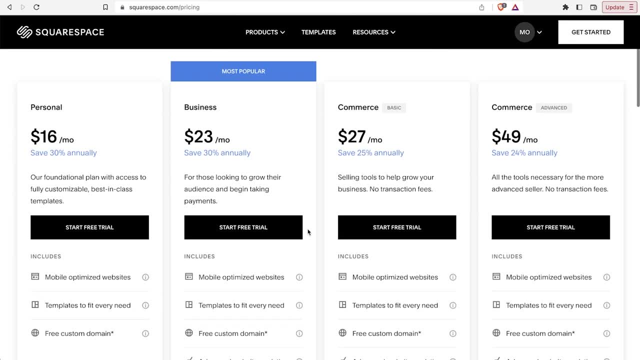 here. you won't be surprised to see it's very similar. There are two strong competitors. Squarespace and Wix are really going at it, But I find that generally Squarespace tends to be slightly more expensive, usually about $1 more per month. But what I really like that they do. 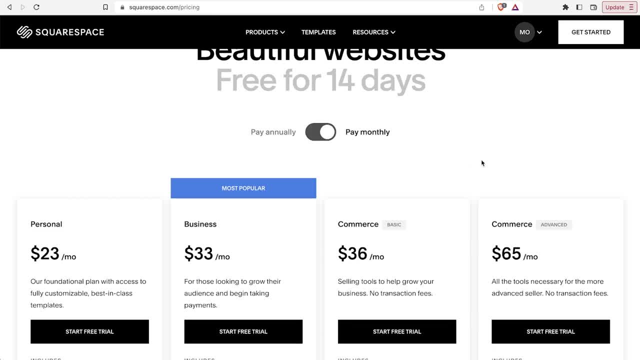 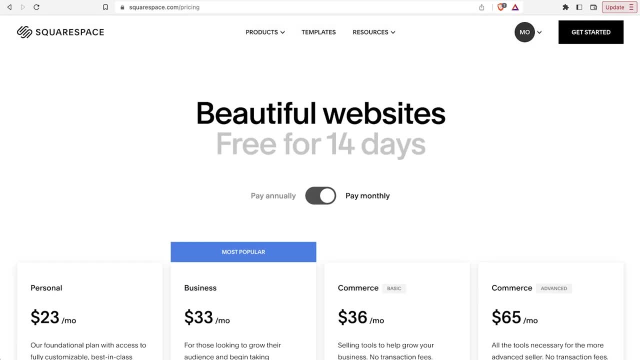 here is: they have this toggle to see what the monthly and annual prices are. Unfortunately, however, they do not have a free plan, So you're gonna have to upgrade no matter what, which I generally recommend for any of these, no matter what you're doing. And then WordPress Now. 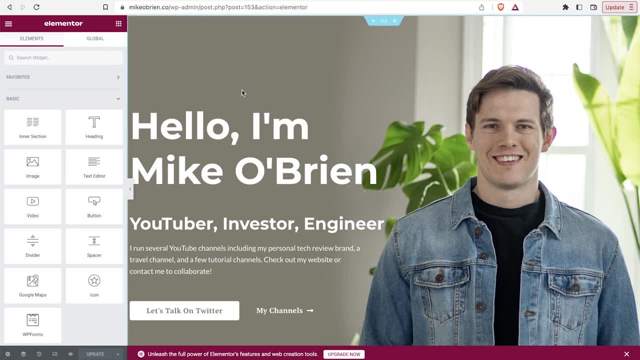 WordPress is actually free to use. Elementor is free to use. WordPress is free to use. It's open source actually, So there's a lot of integrations and a lot of plugins there. That's one of the reasons we like it, And the only thing you'll really have to pay for would be your hosting. 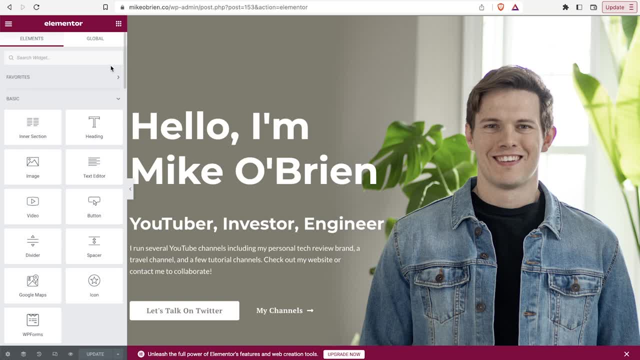 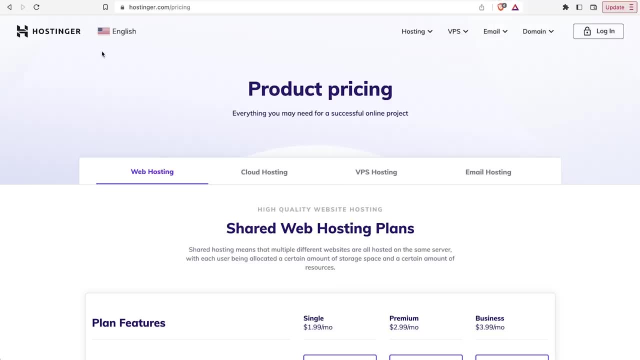 and your domain, unless you want to upgrade, like Yoast SEO, to like a premium version or Elementor Pro, Like you can upgrade things, but the only thing you really need would be your hosting, And so we like to recommend Hostinger: very affordable, super robust, really a solid option. 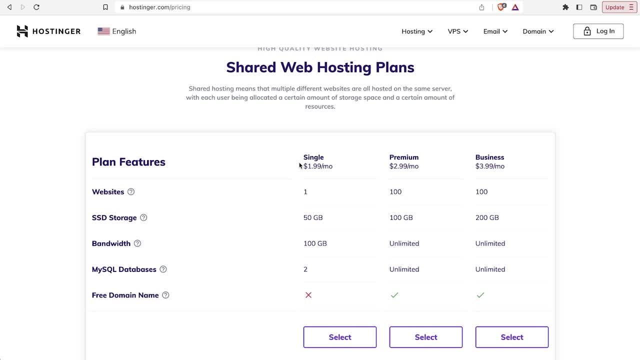 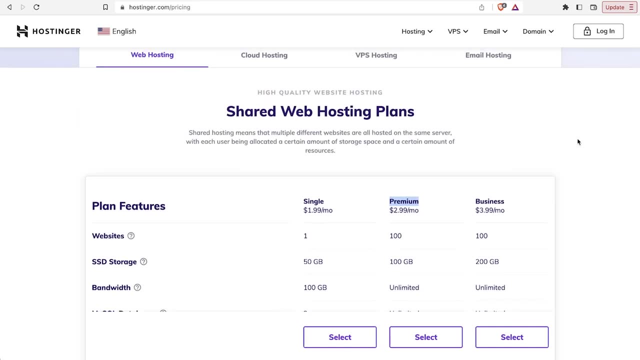 across the board And so you can see just $1.99 a month is their cheapest. plan I usually go with is only $2.99 a month, And then you'll probably pay maybe $10 or $15 per year, which is like a. 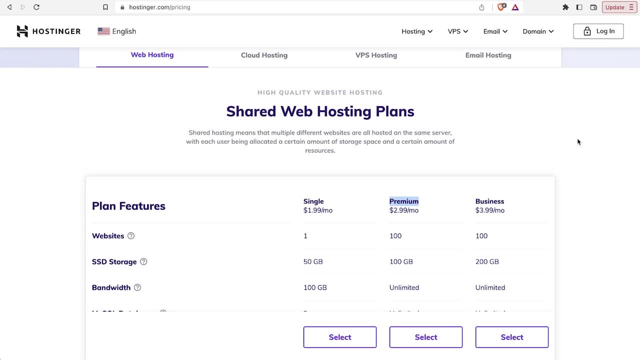 dollar a month for a domain, So overall the most affordable option, well, besides Wix, which is, which is obviously free, like but $3 a month. when you factor in the domain and everything, it's really pretty incredible for hosting a website on one of the most powerful platforms. 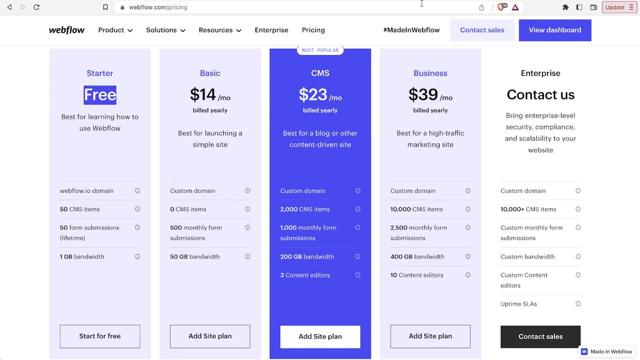 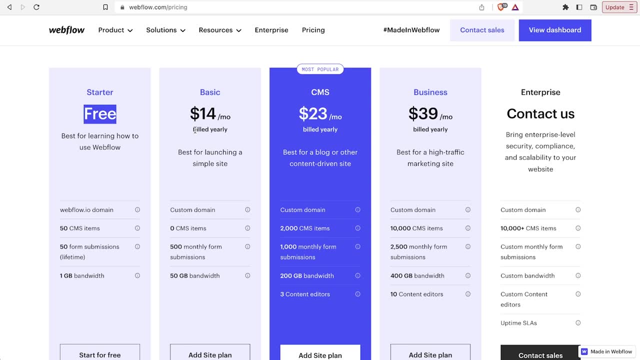 out there. As far as Webflow goes, there is actually a free version which you can use to kind of get started, as you can see right here, And then you'll go up to $14 a month, which is surprisingly- you know it's very reasonable and affordable. Then you can go to. 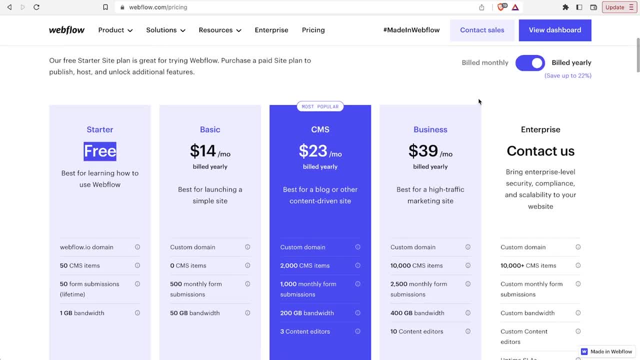 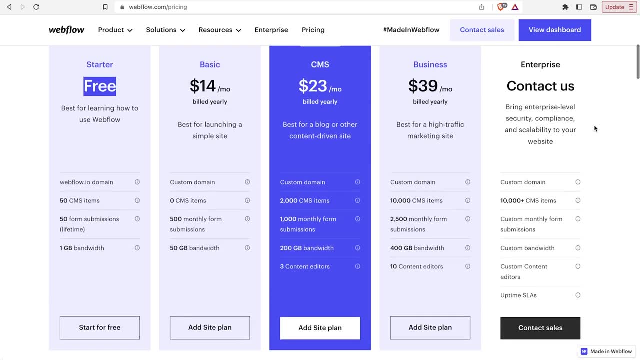 $23 a month. This is billed yearly, though Of course, if you want to pay monthly, got to flip this toggle back And it is a little bit more expensive if you're doing that. And of course, you can go to business or enterprise as well. Obviously, a lot of enterprises would be very happy. 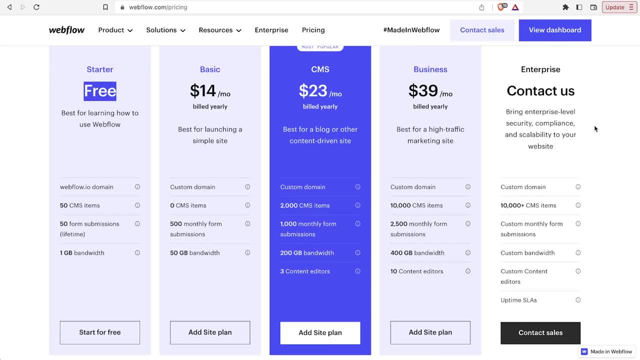 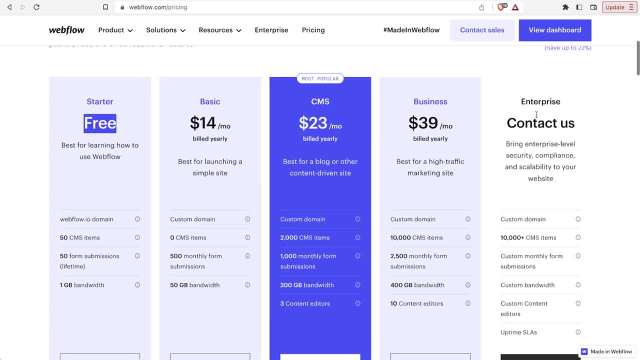 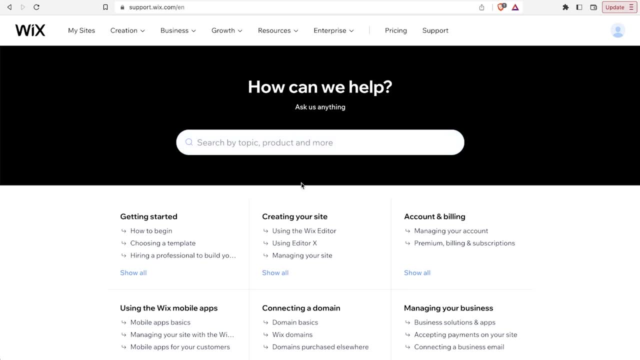 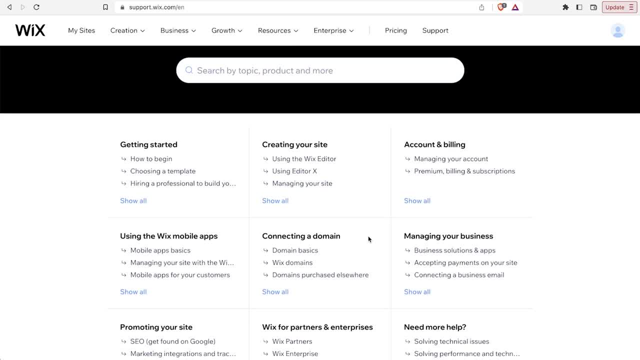 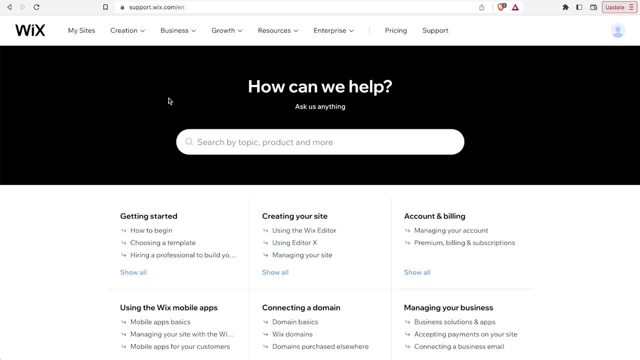 help center that's searchable to answer a lot of the basic questions, but also there is phone and email support And from my experience they've done a really good job helping Squarespace is pretty similar. They also have a help center, a live chat and email support. WordPress is a little. 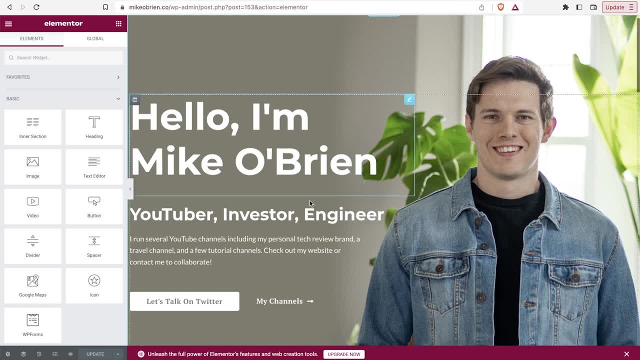 bit trickier. So WordPress, like I said, it's a little bit more complex. it's a little bit more complicated, but it's a little bit more fun to use. So I think it's definitely worth a try. WordPress: like I said, it's free to use WordPress, so you can't really expect them to. 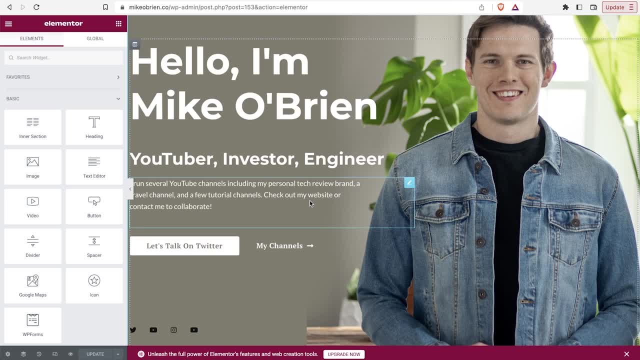 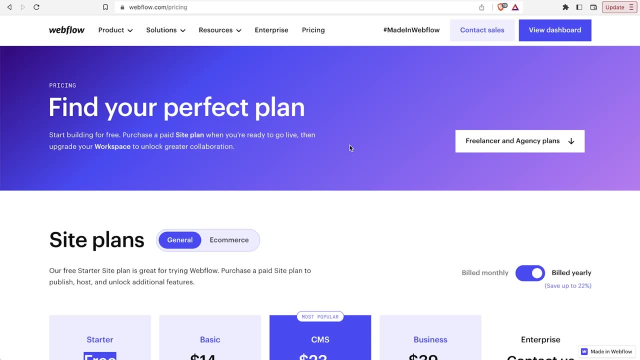 help, But there is a really big community, a lot of forums and there are some different official supports- for WordPress, probably, And then, of course, Webflow has their own help center, their own email support and some forums as well. Alright, so that's my comparison between the four. 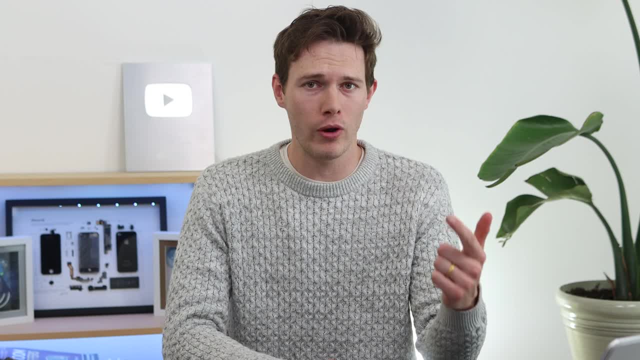 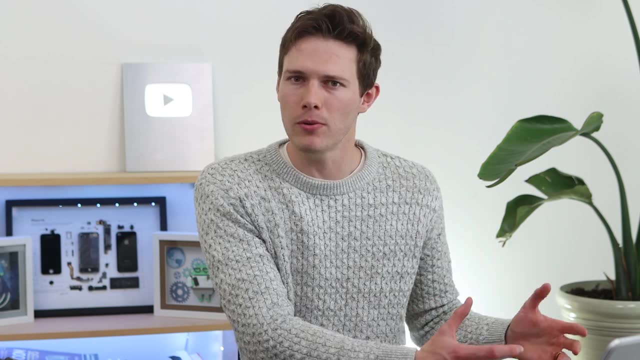 most popular website building tools out there: Wix, Squarespace, Webflow and WordPress. To summarize, Wix is great for anything from a single page website, a simple little one, all the way up to a single page website. So if you're looking for a single page website, 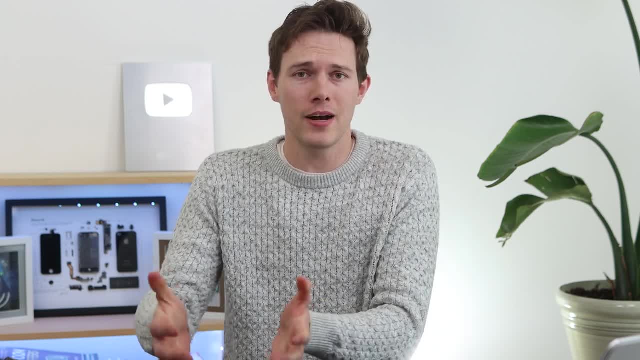 Wix is great for anything from a single page website, a simple little one, all the way up to a more advanced, even professional, website that an enterprise or a larger business would use. You could really use it at any size. It's easy to blog. It's great for selling things. 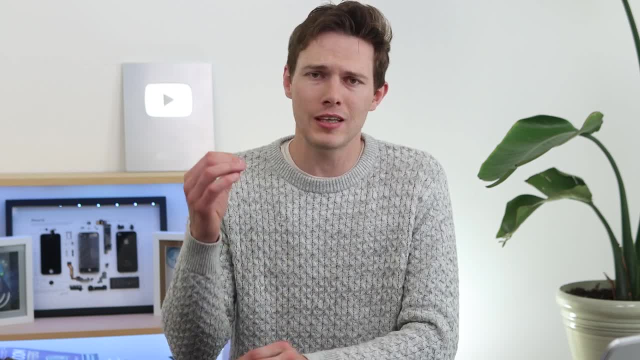 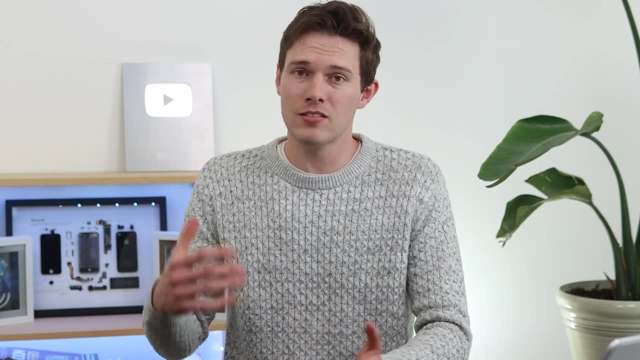 really great for customizing with very little effort and choosing exactly what you want. So Wix: super solid recommendation for pretty much anybody out there. Then Squarespace really goes head to head with Wix. They have a lot of customization now with. 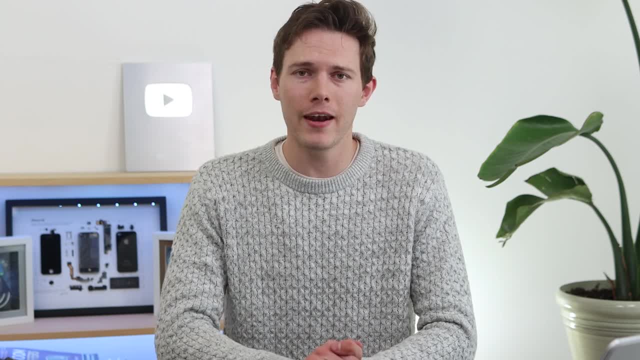 their new layout on how they can design the website with the drag and drop editor, And on top of that you still have a lot of customizations. So if you're looking for a single page website, you still have a lot of really good fundamental things on there: The ability to host podcasts. 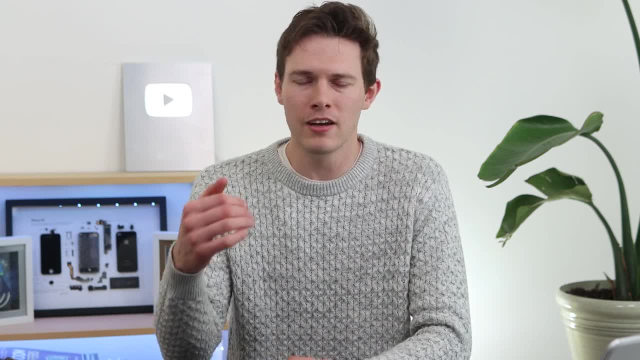 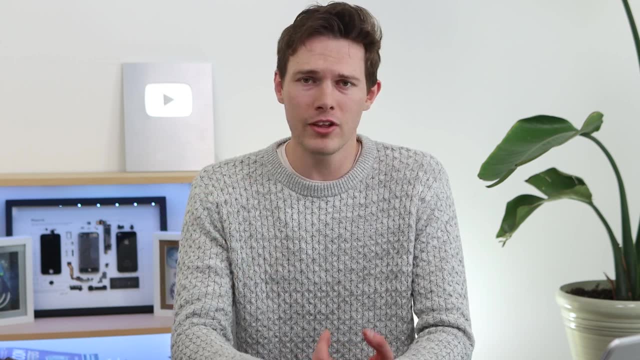 for example, everything baked in. There's not as many plugins, but you don't necessarily need the plugins, because Squarespace offers most of that functionality already baked in. You can sell things on there You can schedule for, like a local doctor's office or a restaurant or whatever. 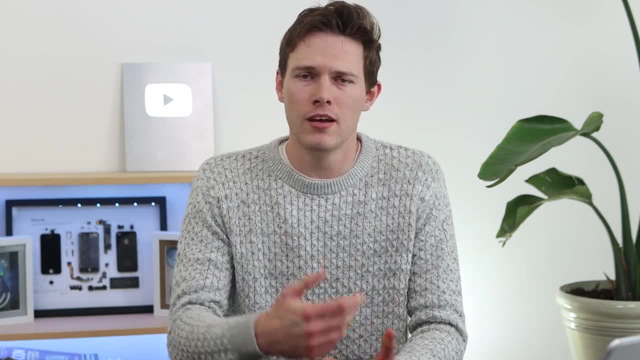 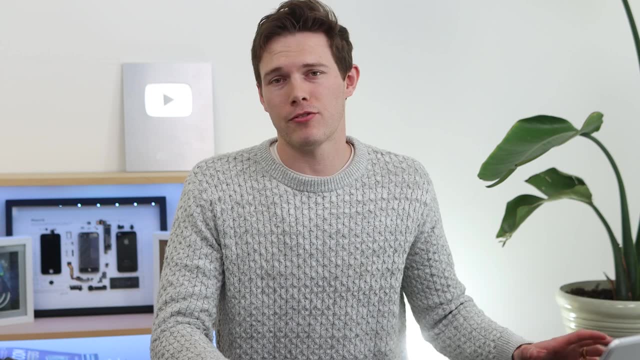 You can sell things like takeout if people want to order from your restaurant. Very flexible, but it doesn't like it keeps it very simple in the interface. And then we have WordPress, kind of the opposite of the first two rather than being very refined and easy to use. 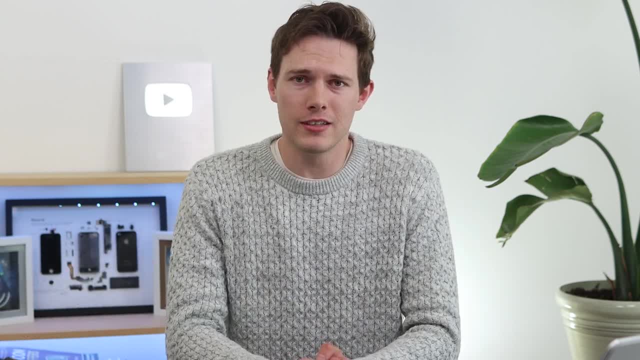 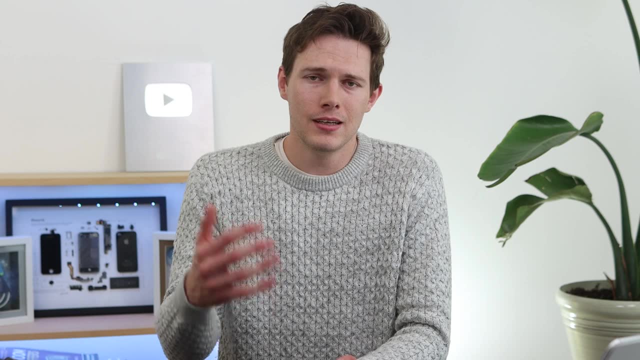 It really has an ocean of options and you can do a lot with this, but it does take a lot more research. It's incredibly powerful and there's a reason- it powers one third of the internet, but it takes more learning. Then, of course, we have Webflow. 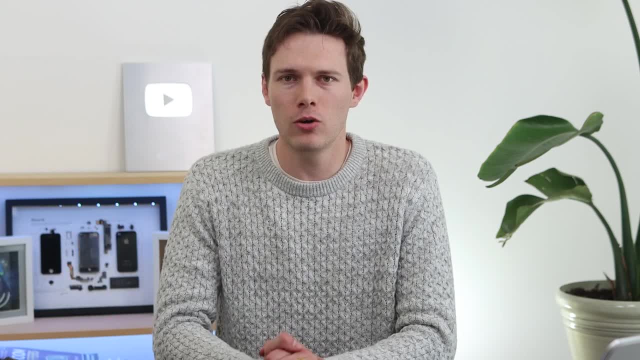 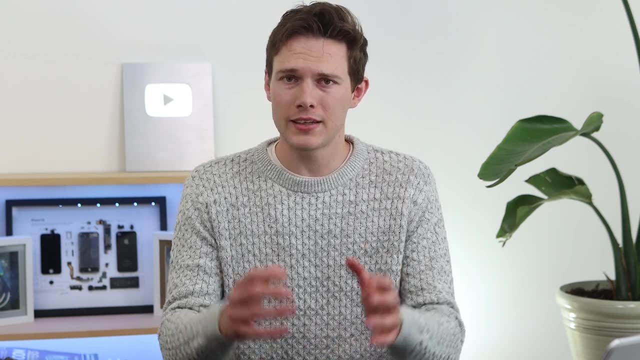 which is kind of a unique one. It's very much in the class of its own, in that you can add custom animations and really do a lot of more advanced design and even do some coding on there as well, while keeping it kind of a balance between hardcore, like full stack developer, and the